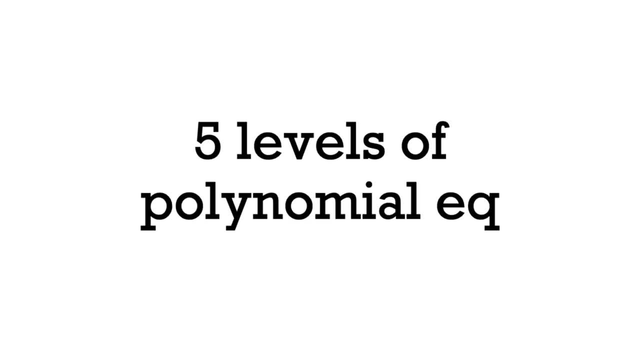 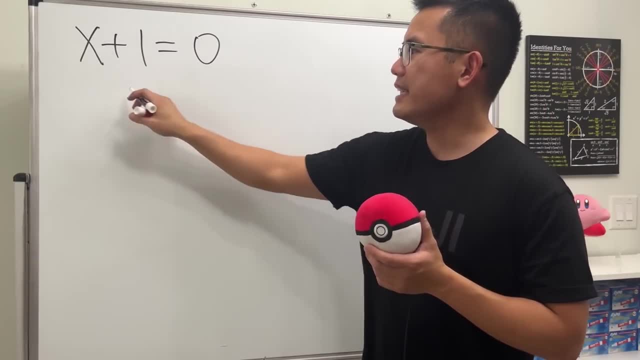 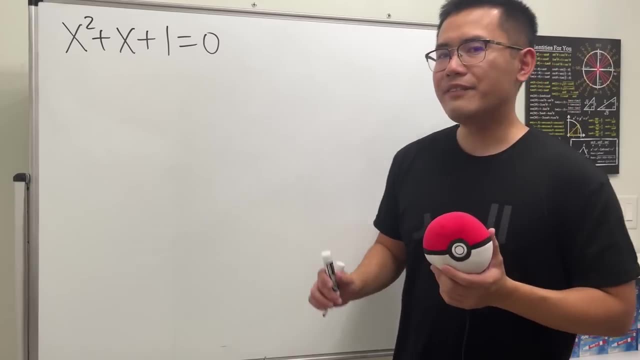 Five levels of polynomial equation. Level one: Here we have this linear equation: x plus one equal to zero. We can just move the one to the other side and we get x is equal to negative one, and then we are done Good. Level two: So now we have a quadratic equation: x squared plus x plus. 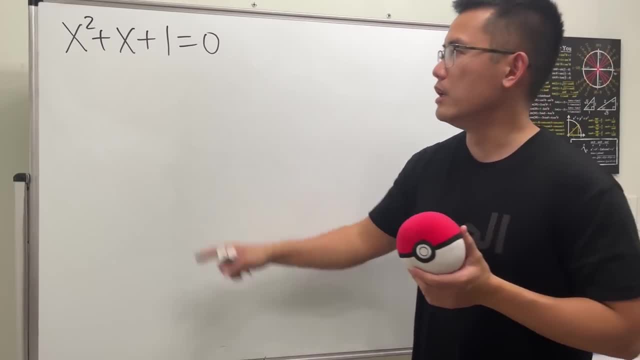 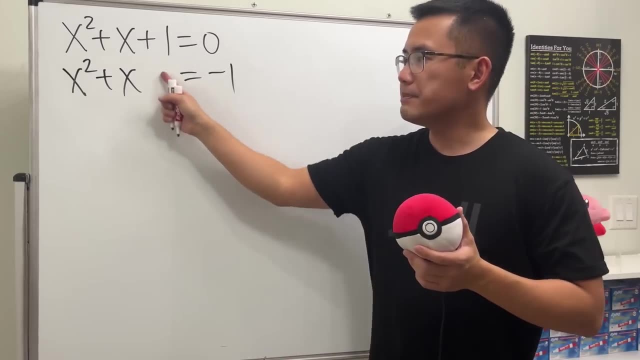 one is equal to zero. Well, let's go ahead and do this by completing a square. First move the one to the other side, so we will have x squared plus x, and then that's equal to negative one. And for this part, right here we are going to find the magic number so we can complete the square And 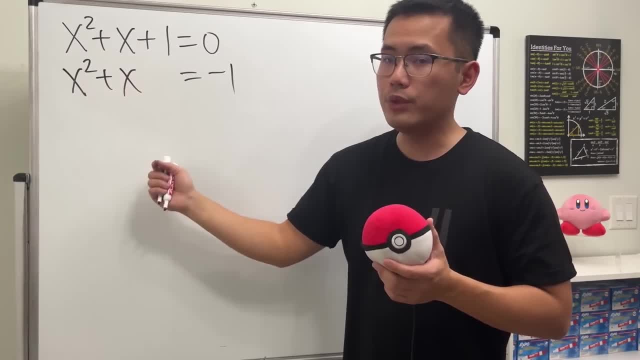 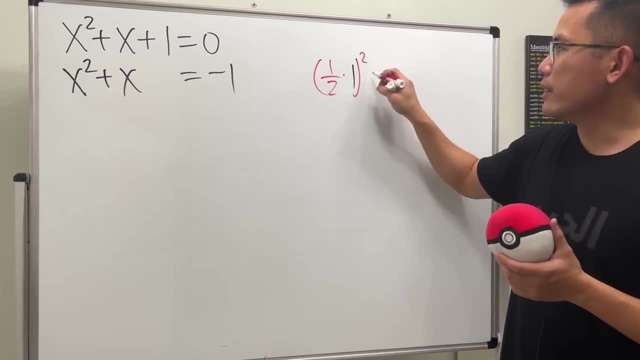 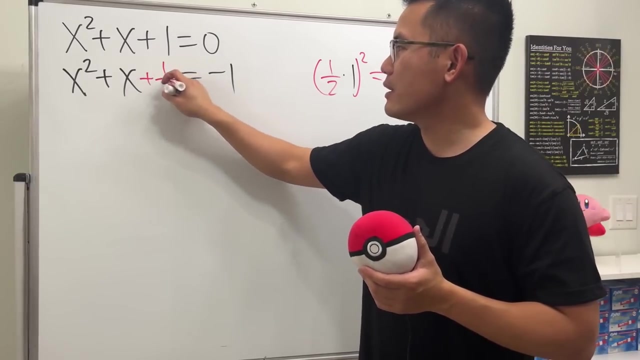 to do so, we first make sure that we have a one in front of x squared, which we do. Then we see the coefficient of x, which is one, and we will have to take half of that and then square, Work this out. we will get one over four. So this is the magic number. Now we have to add on both sides here. 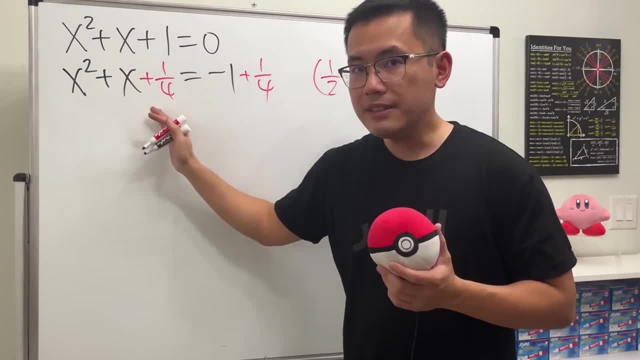 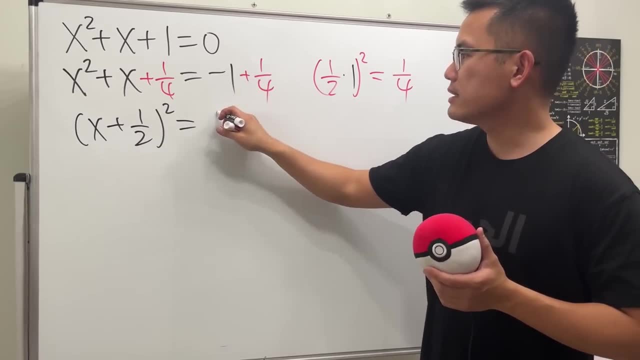 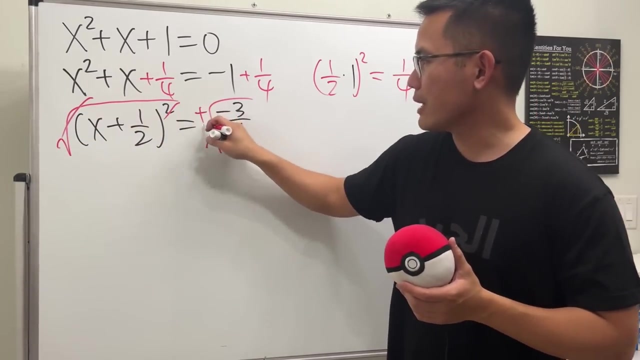 and here. So the left hand side is going to give us x plus one half square, and then on the right hand side, this is going to give us negative three over four. Now we can just take the square roots on both sides, Cancel this out and then put on the plus or minus. On the left hand side, we get x plus one. 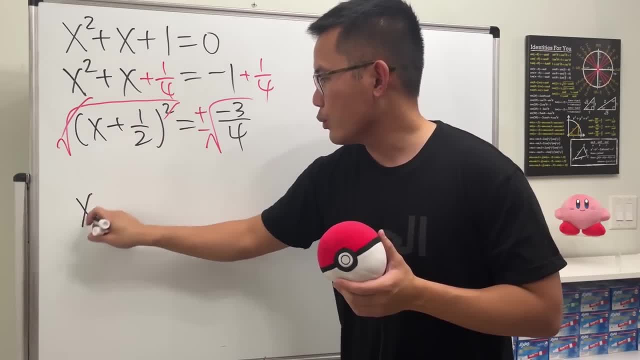 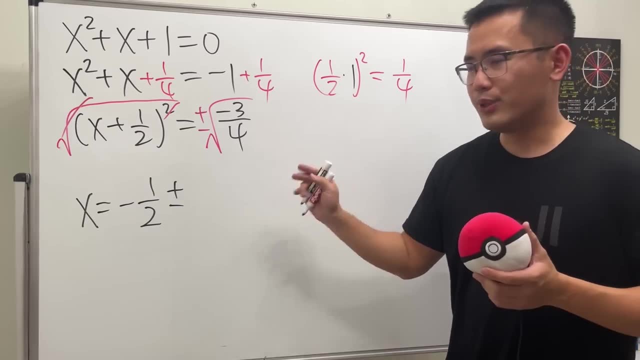 half, But let's move the one half to the other side. So x will be equal to negative. one over two plus or minus. square root of four is just a two on the bottom, And then we have square root of negative, which is going to be the i, and then the three right still. 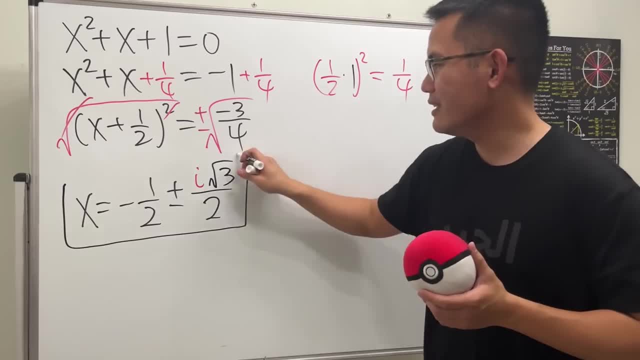 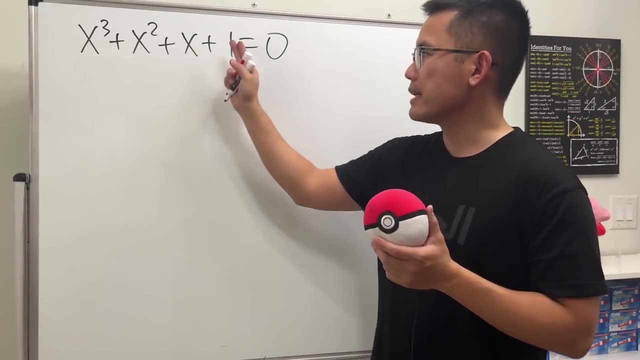 inside the square root. So, ladies and gentlemen, this, right here is it. Great. Level three. And now for this cubic equation: x cube plus x, squared plus x plus one is equal to zero. We don't have to use the cubic formula, We can actually just do this by factoring. Check this out, I'm going to. 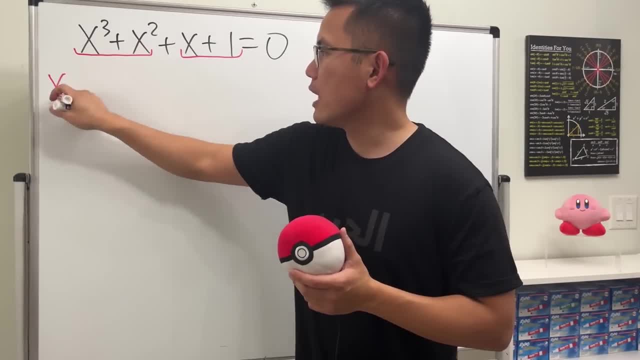 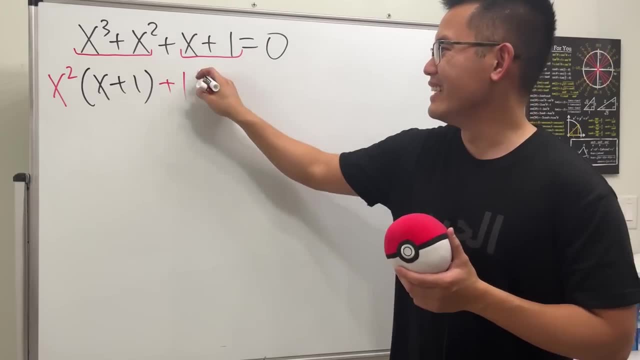 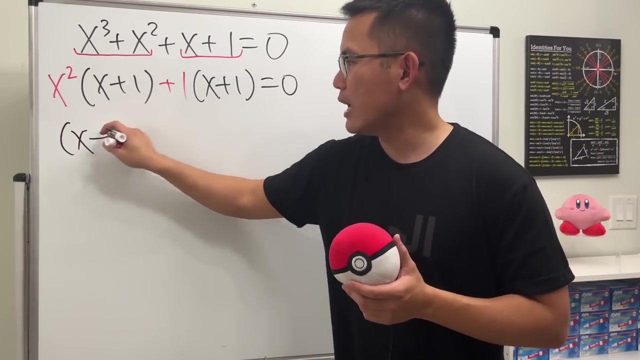 do it by grouping For these two terms. we can factor out the x squared, and then we will just get x plus one For these two terms. we can just factor out like a one, like this, and then we still have that x plus one, and the nice thing is that the x plus one is in common. so we can factor that out like this and: 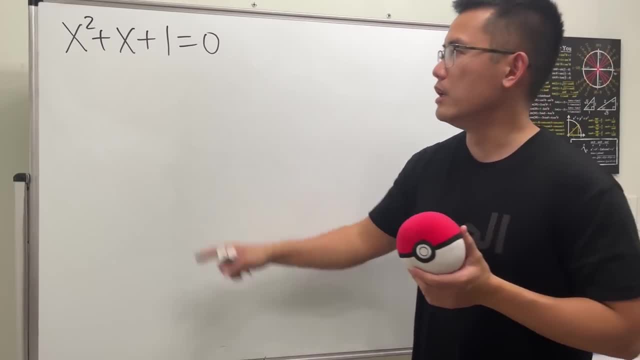 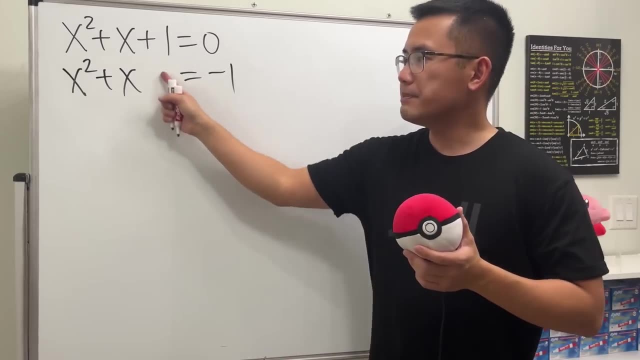 one is equal to zero. Well, let's go ahead and do this by completing a square. First move the one to the other side, so we will have x squared plus x, and then that's equal to negative one. And for this part, right here we are going to find the magic number so we can complete the square And 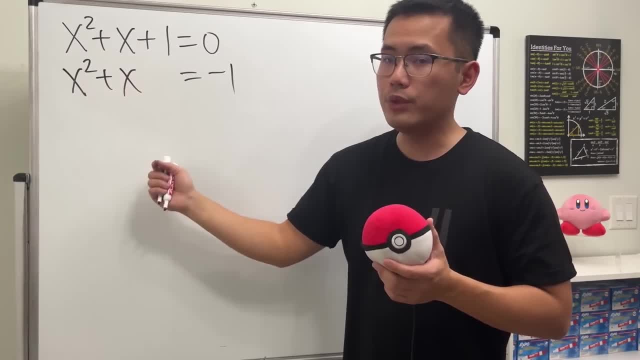 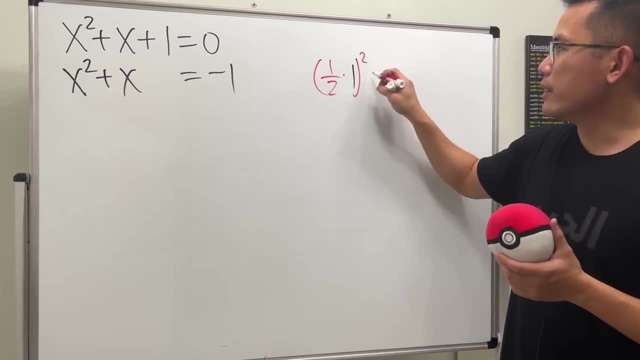 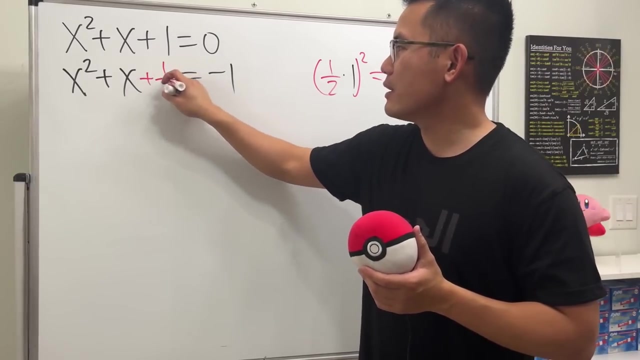 to do so, we first make sure that we have a one in front of x squared, which we do. Then we see the coefficient of x, which is one, and we will have to take half of that and then square, Work this out. we will get one over four. So this is the magic number. Now we have to add on both sides here. 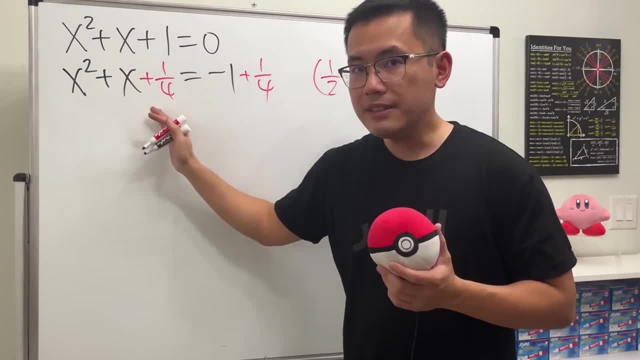 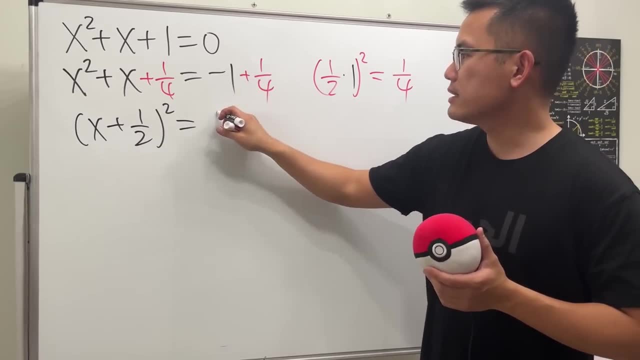 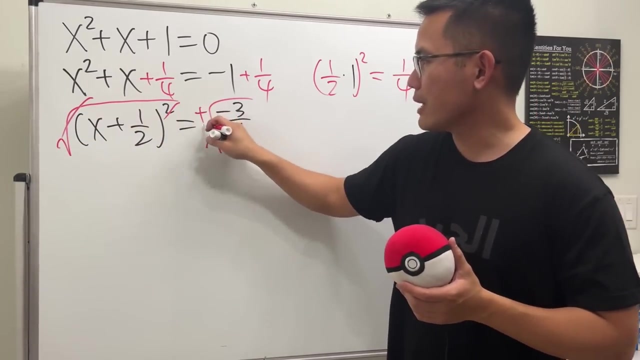 and here. So the left hand side is going to give us x plus one half square, and then on the right hand side, this is going to give us negative three over four. Now we can just take the square roots on both sides, Cancel this out and then put on the plus or minus. On the left hand side, we get x plus one. 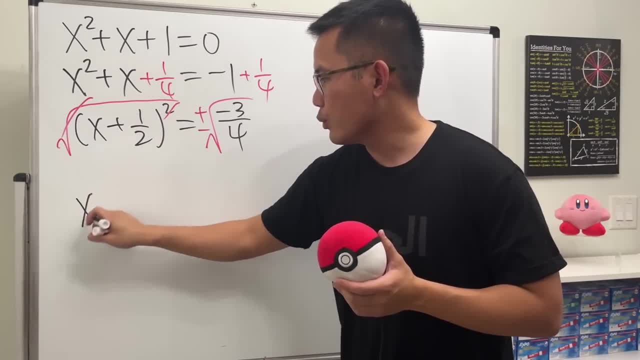 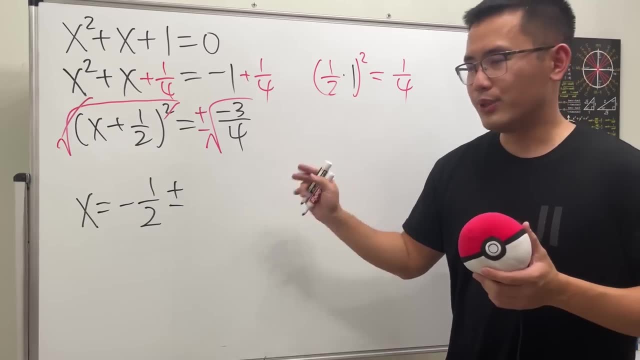 half, But let's move the one half to the other side. So x will be equal to negative. one over two plus or minus. square root of four is just a two on the bottom, And then we have square root of negative, which is going to be the i, and then the three right. 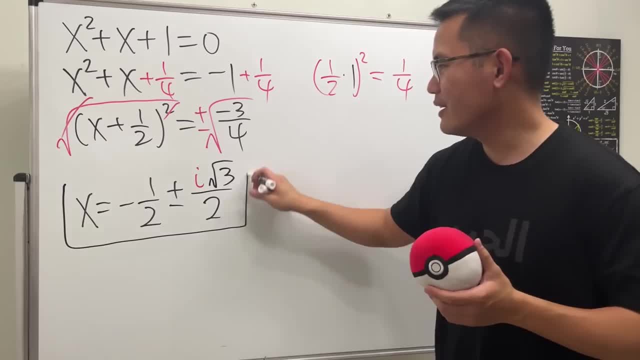 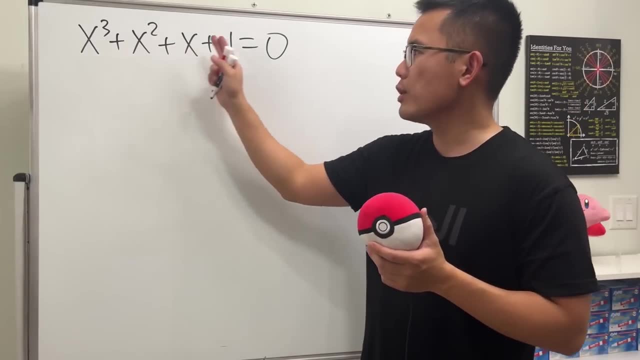 still inside the square root. So, ladies and gentlemen, this, right here is it. Great. Level three. And now for this cubic equation: x cube plus x square plus x plus one is equal to zero. We don't have to use the cubic formula, We can actually just do this by factoring. Check this out. 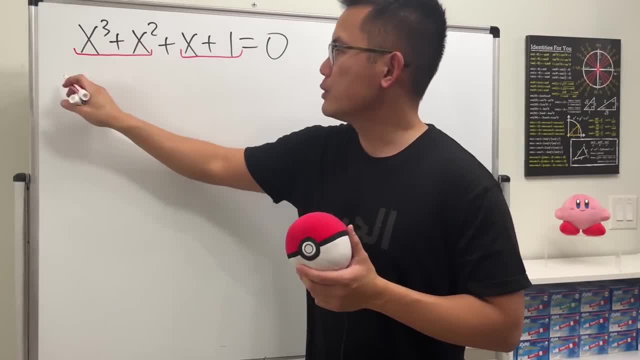 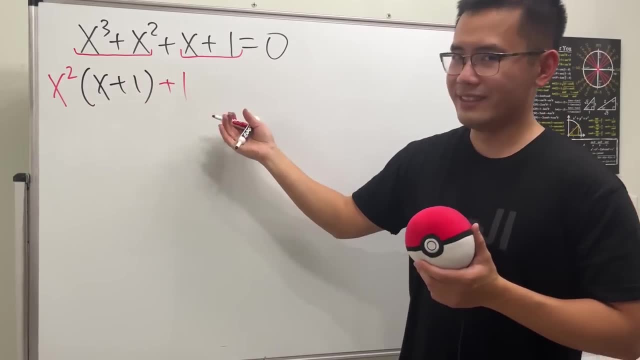 I'm going to do it by grouping. For these two terms, we can factor out the x squared, and then we will just get x plus one. And for these two terms we can just factor out like a one, like this, And then we still have that. 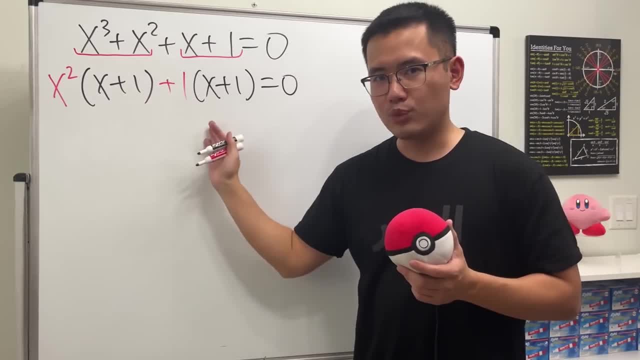 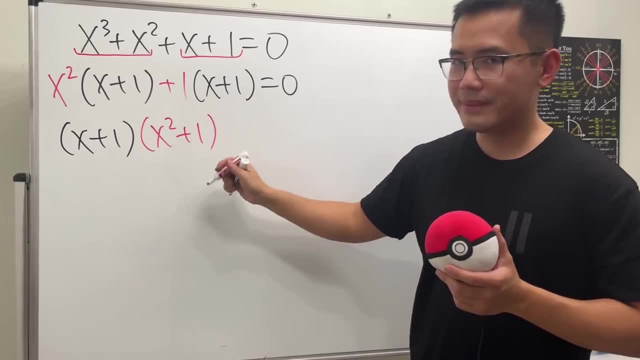 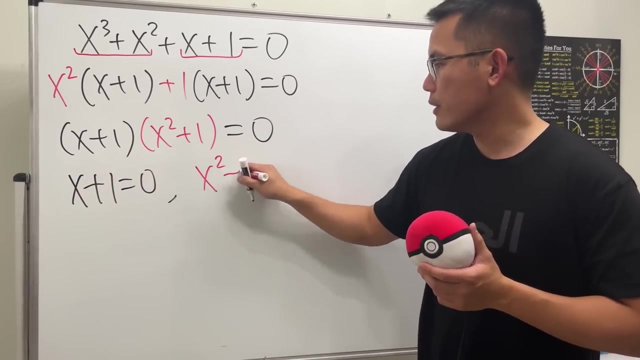 x plus one, And the nice thing is that the x plus one is in common, So we can factor that out like this, And then we will have that x squared plus one left, And this is still equal to zero. Now put this to be zero, And we also have to put this to be zero. So we see that right here. just move the. 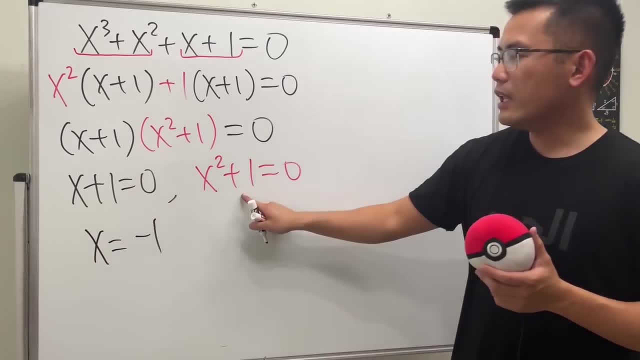 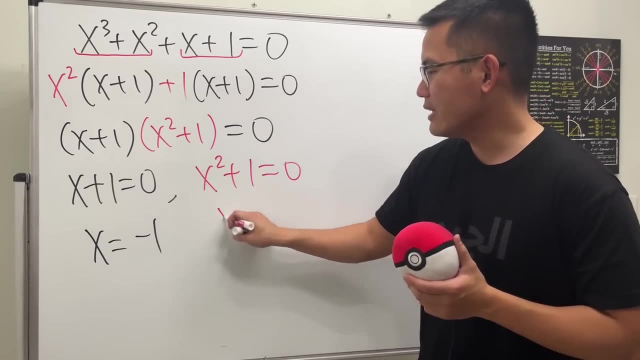 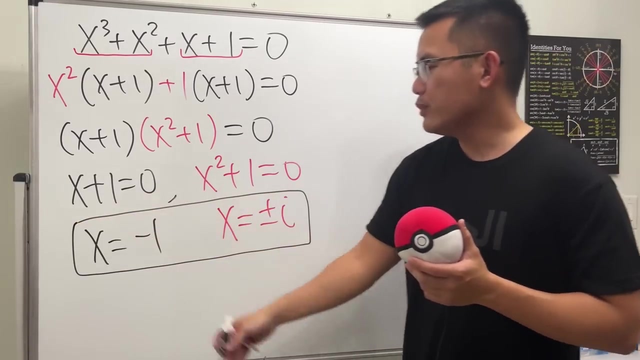 one to the other side, X will be equal to negative one. And right here we can move the one to the other side and take the square roots on both sides. And don't forget the plus or minus. Right here we can get: x is equal to plus or minus i. So we have a total of three answers: Negative one. 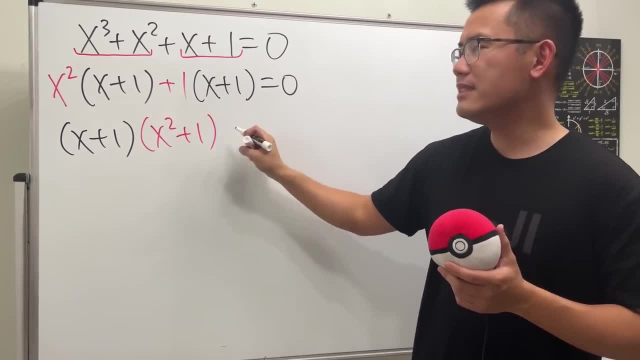 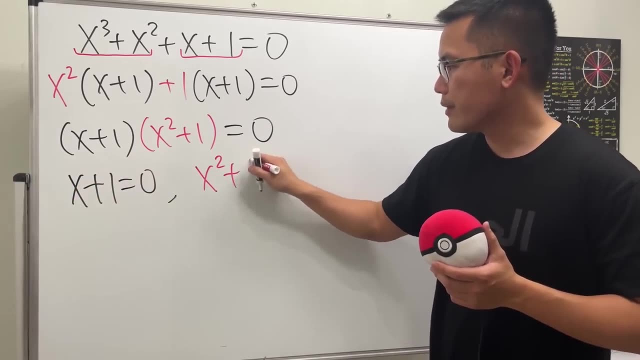 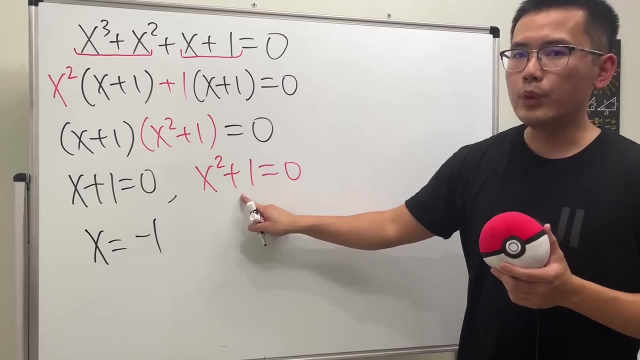 then we will have that x squared plus one left, and this is still equal to zero. Now, put this to be zero, and we also have to put this to be zero. So we see that, right here, just move the one to the other side. x will be equal to negative one, and right here we can move the one to the. 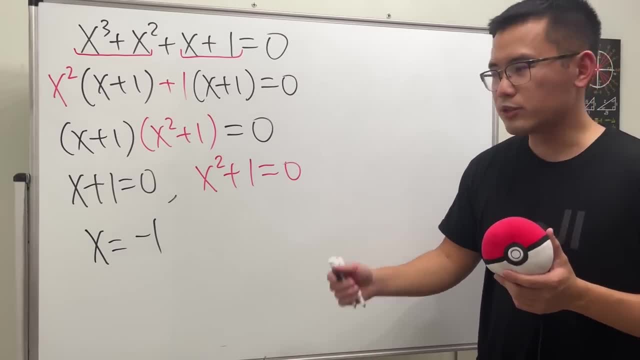 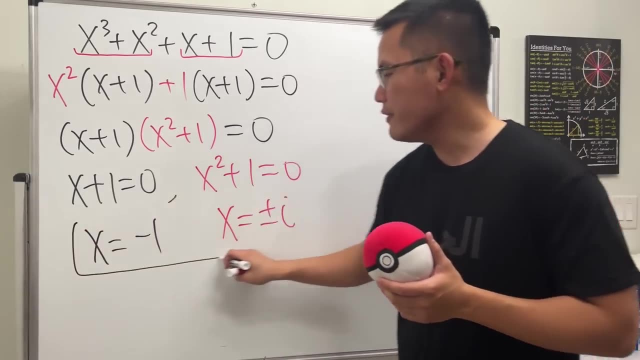 other side and take the square roots on both sides, and don't forget the plus or minus right here we can get: x is equal to plus or minus i. So we have a total of three answers: negative one and the i, and also the negative i Nice. 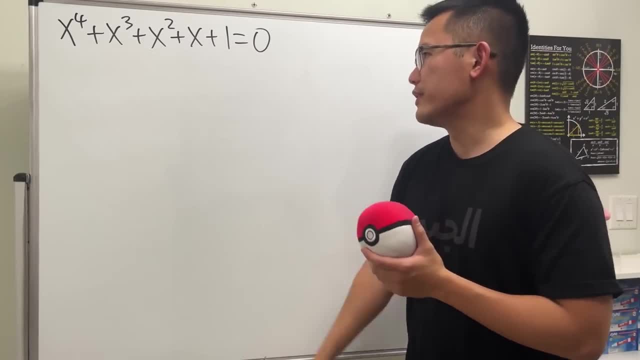 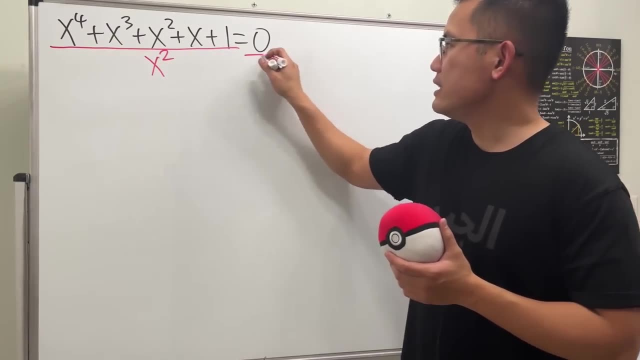 Level four. And now we have this quadratic equation. What do we even do? The quadratic formula? No, don't do that. Check this out. We are going to divide everybody by x squared, and you will see that this will work out very nicely. 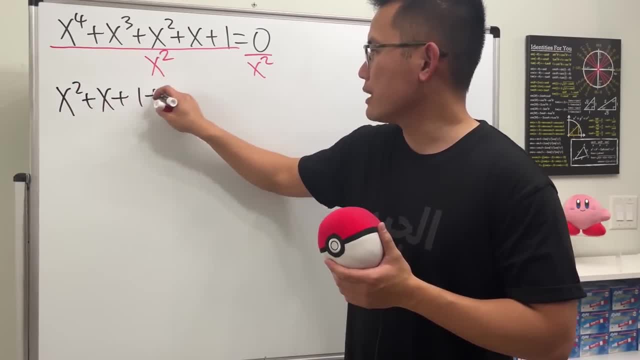 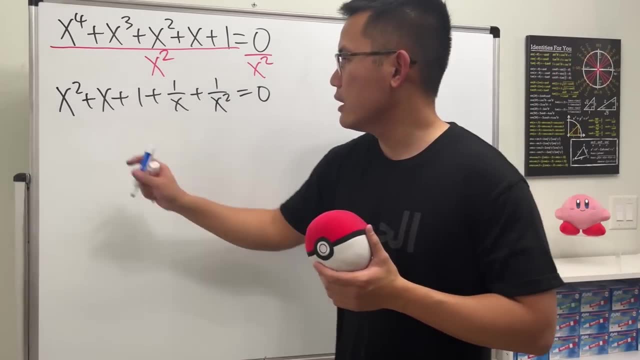 So if we divide them individually, we get x squared plus x plus one plus one over x, plus one over x squared, and that's equal to zero. Now focus on the x squared plus one over x squared, because in fact we can complete a square for them. 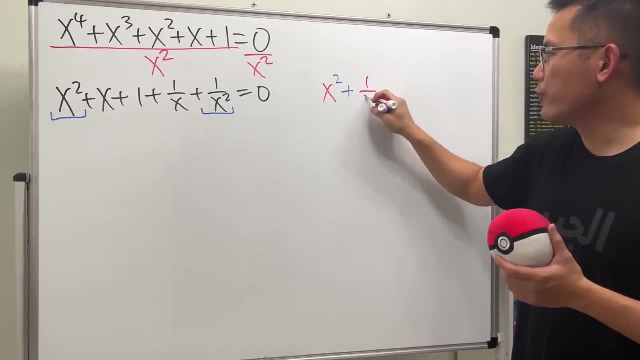 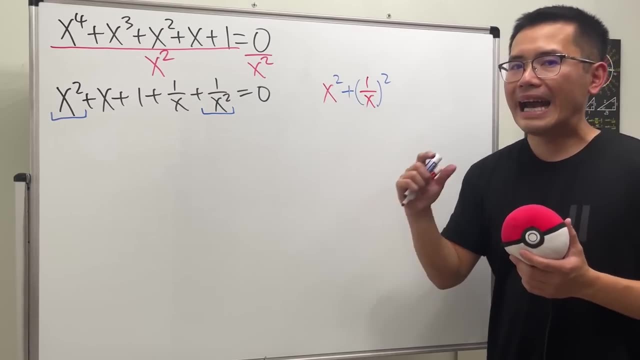 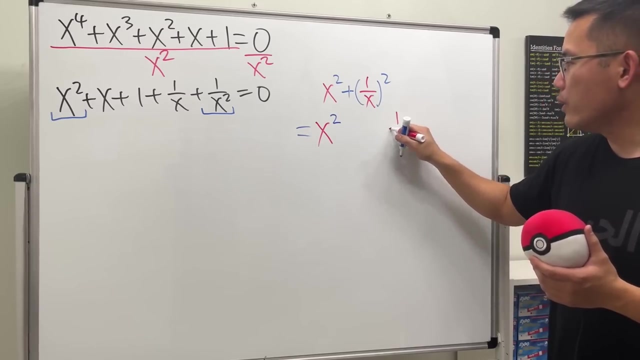 Right here I'm going to write down. we have x squared plus one over x and then square. This is the sum of two squares. We can complete a square by adding a middle term and the middle term is the first. we have that x squared and then this right here is that one over x and then squared. 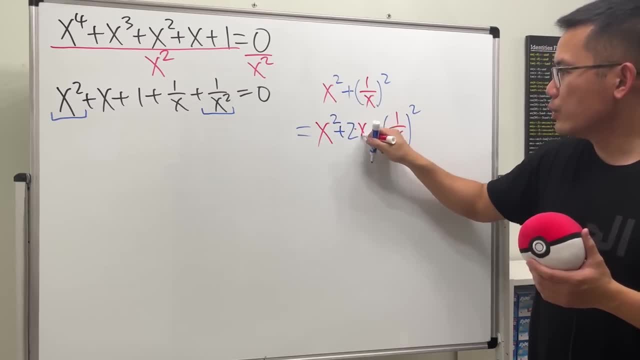 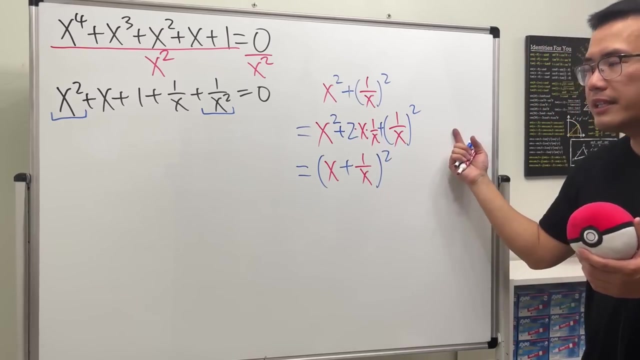 If we add two times this and that, which is actually just a number two, Right this right here, will give us the perfect square named the x, plus one over x, and then squared. Very nice, But of course, if we added this term, we will have to subtract it, and this is technically just one. 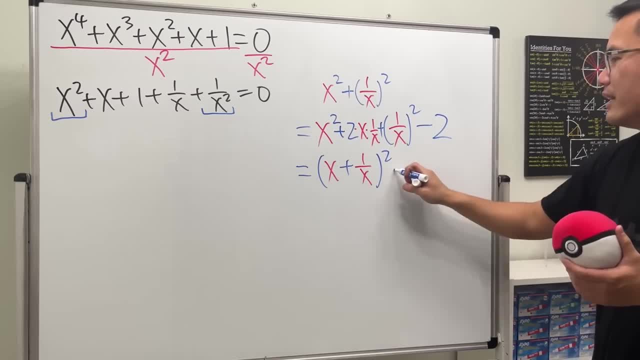 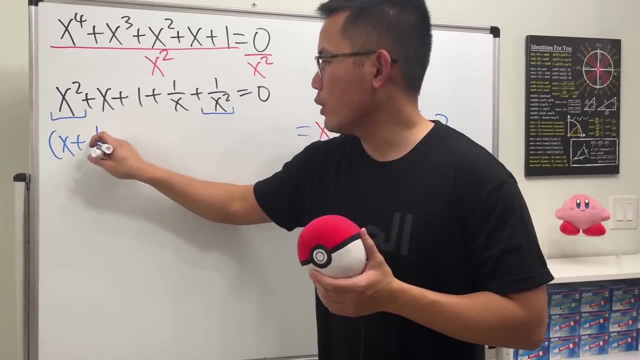 two. right, it's just a number two. so we just have to minus two at the end, like so. So we just have to minus two at the end, like so, so. So now for this, and that I'm going to replace it with this, so we have parentheses x plus 1 over. 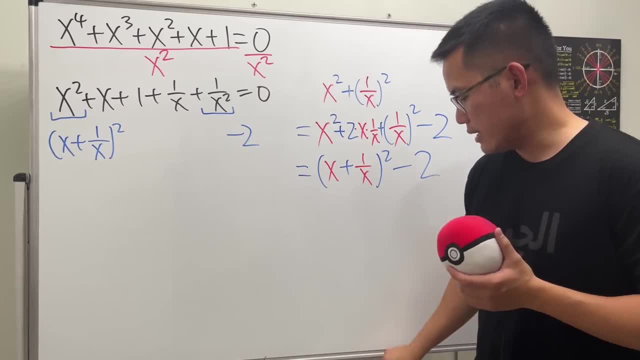 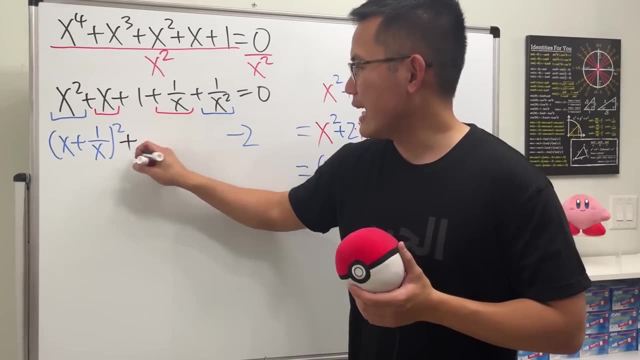 x and then square, and let me just put a minus 2 all the way at the end right here, and then we have this x plus 1 over x as well. Very nice, huh. So let's go and add x plus 1 over x and then of. 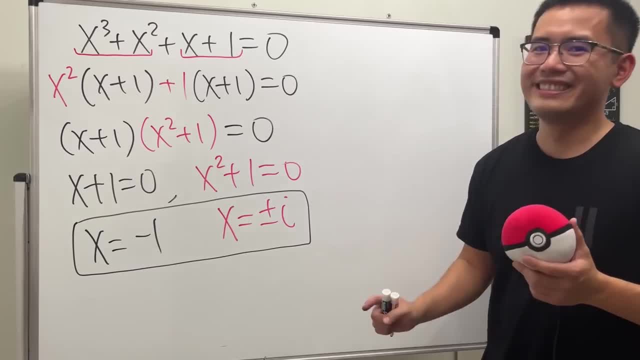 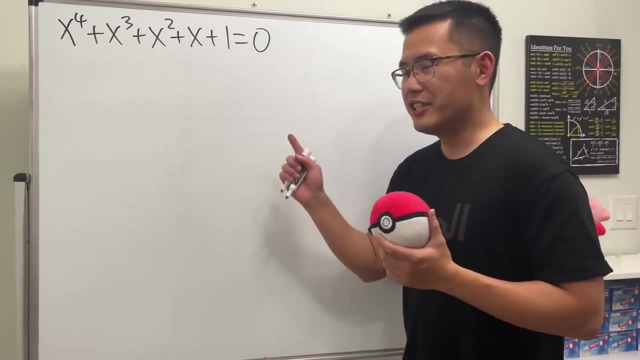 and the i, and also the negative i, Nice, Level four. And now we have this quadratic equation. What do we even do? The quadratic formula? No, don't do that. Check this out. We are going to divide everybody by x squared, And you will see that this will work out very nicely. Split it and 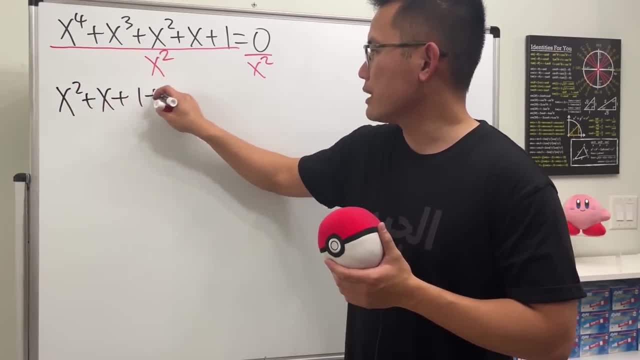 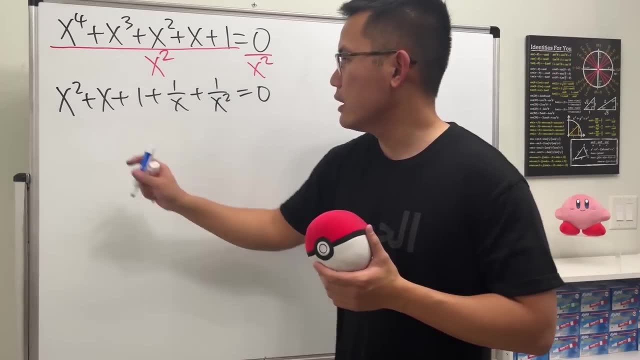 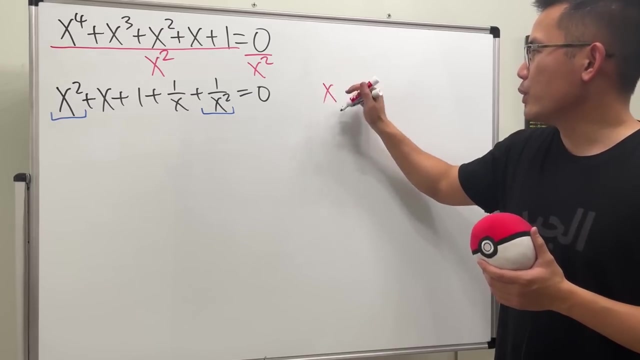 them individually, we get x squared plus x plus 1 plus 1 over x plus 1 over x squared, and that's equal to 0.. now focus on the x squared plus 1 over x squared, because in fact we can complete a square for them right here. i'm going to write down: we have x squared plus 1 over x and then square. 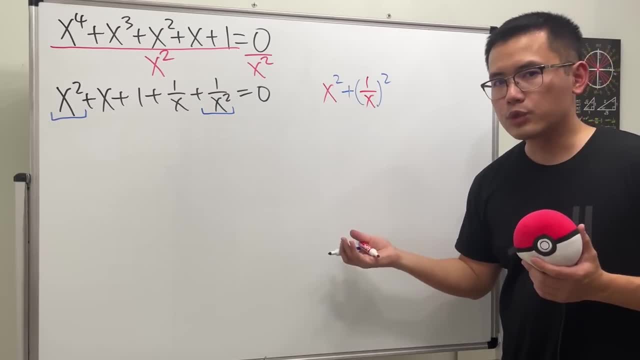 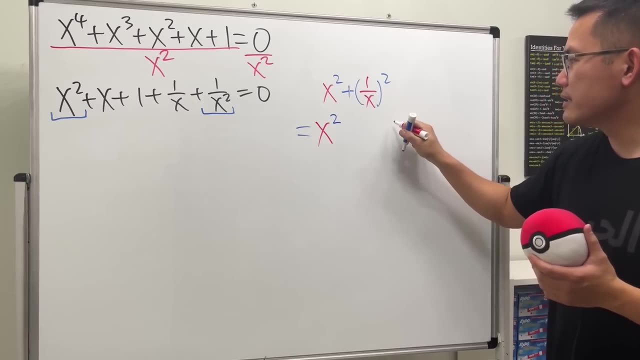 this is the sum of two squares. we can complete a square by adding a middle term, and the middle term is the following: first we have the x square and then this: right here is that 1 over x and then square if we add 2 times this and that, which is actually just a number 2. right this, right here. 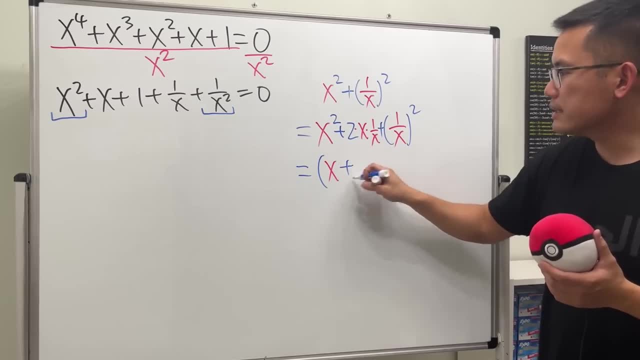 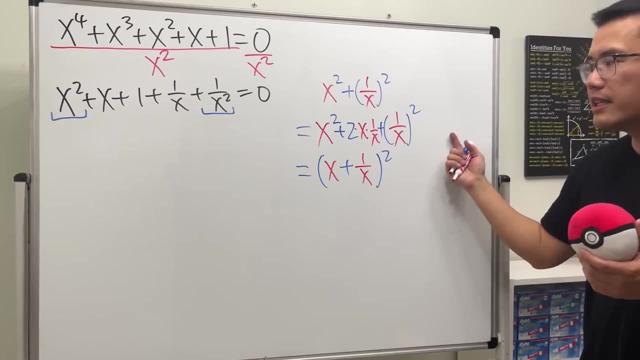 will give us the perfect square named the x plus 1 over x and then square. very nice, but of course, if we added this term, we will have to subtract it, and this is technically just one, two, right, it's just a number two, so we just have to. 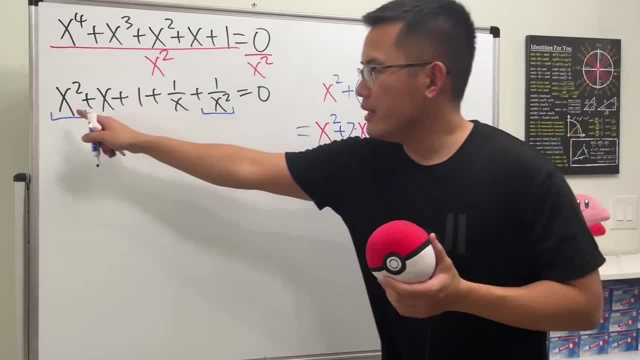 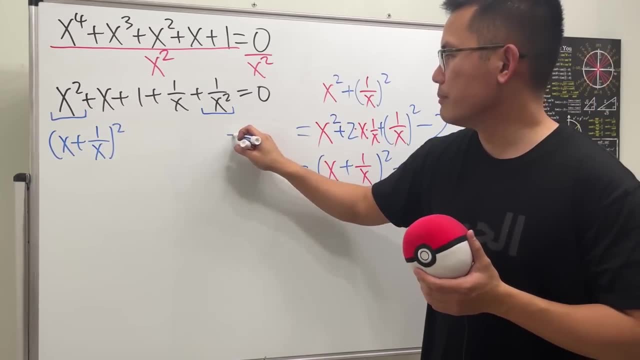 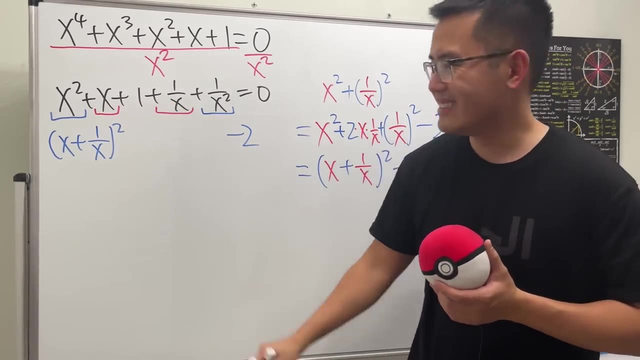 minus 2 at the end, like so. so now for this, and that i'm going to replace it with this. so we have parentheses, x plus 1 over x, and then square, and let me just put a minus 2 all the way at the end, right here, and then we have this x plus 1 over x as well. very nice, huh. so let's go and add x plus 1. 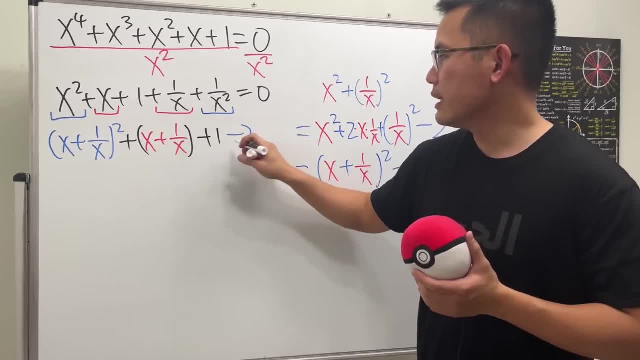 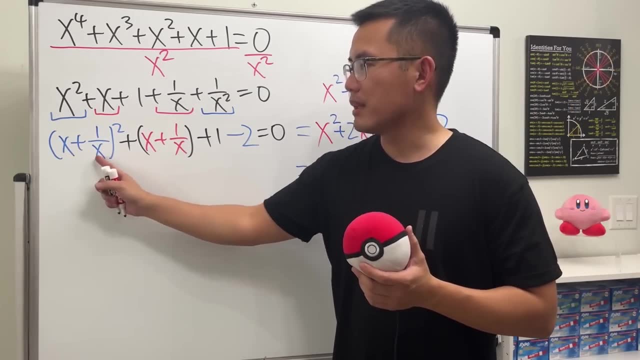 over x, and then, of course, we still have that plus 1 and minus 2, and that's equal to 0.. in fact, we can just do this, and we can just do the same thing, but in terms of x plus 1 over x. so now let's just 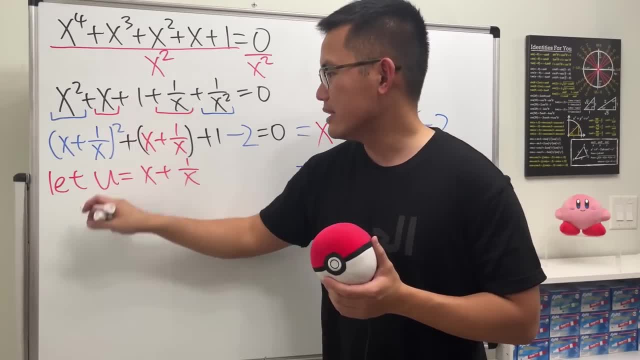 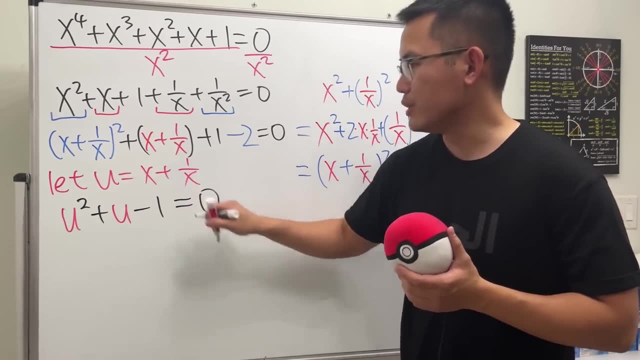 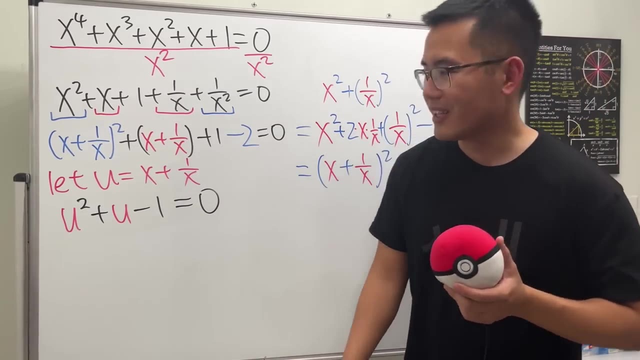 do a new substitution, that u equal to x plus 1 over x, because this way we can see that this is u square plus u and then this is just minus 1 and that's equal to 0, and because earlier we use the method of completing a square. so right now let's solve this by using the quadratic formula. so u is 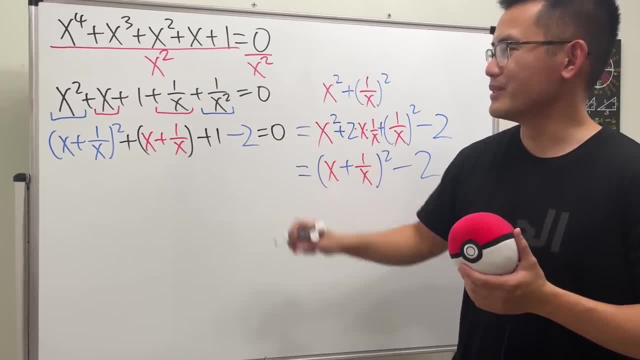 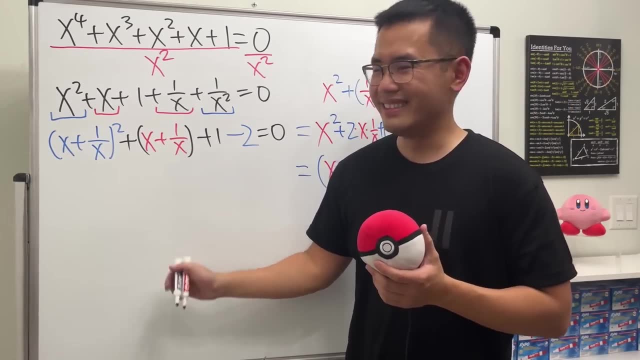 course we still have that plus 1 and minus 2, and that's equal to 0.. In fact we have a quadratic equation in terms of x plus 1 over x. So now let's just do a u-substitution: let u equal to x. 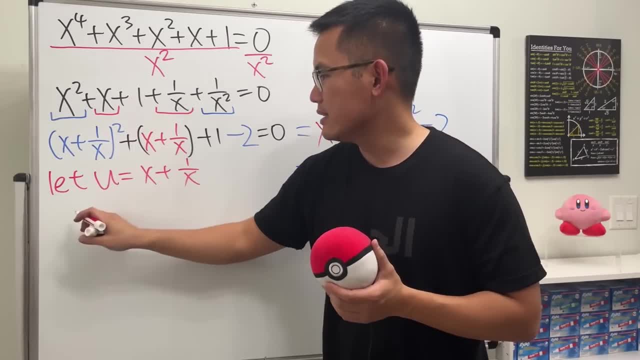 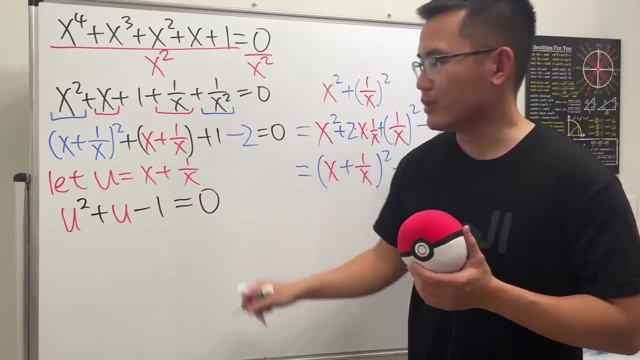 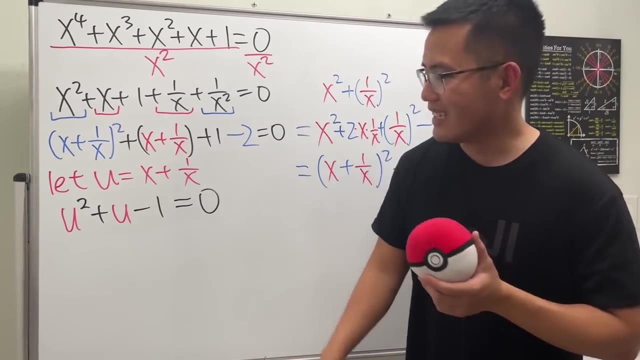 plus 1 over x, because this way we can see that this is u squared plus u, and then this is just minus 1, and that's equal to 0.. And because earlier we used the method of completing a square, so right now let's solve this by using the quadratic formula. So u is equal to negative 1. 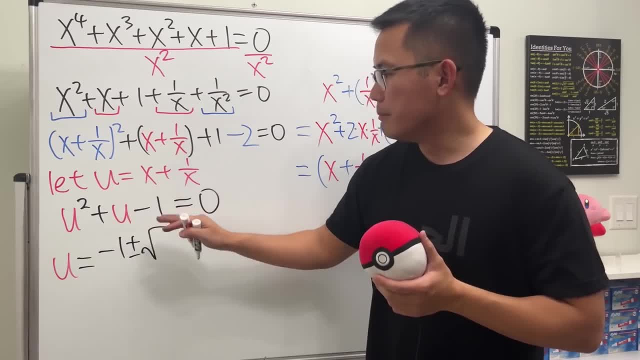 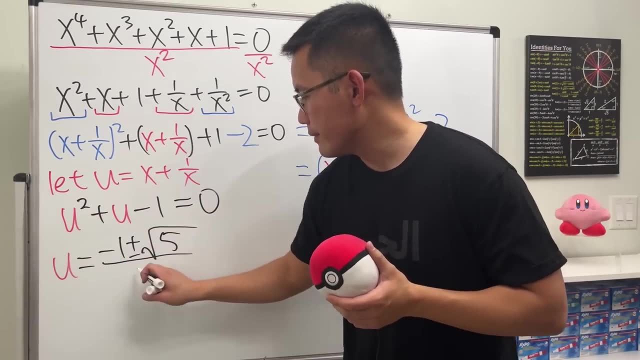 plus 1 over x, and that's equal to 0.. So let's solve this by using the quadratic formula: So minus square root of 1, square minus 4 times this and that which is going to be plus 4, so to get this 5, and then all over 2 times 1.. Cool, You know what's cooler? This right here. 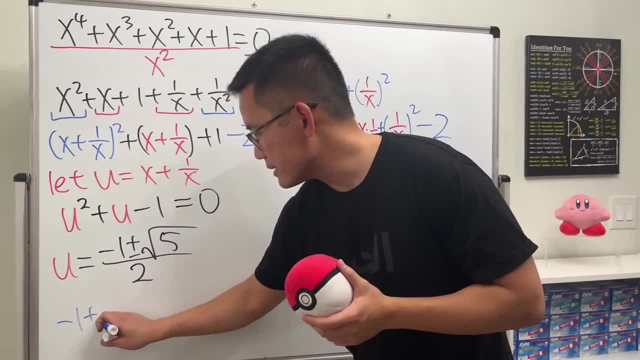 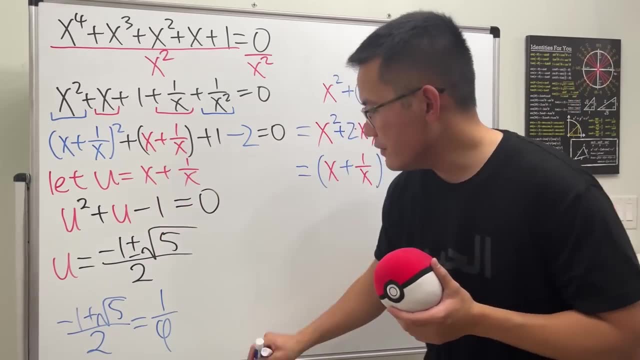 when we take the positive, negative 1 plus square root of 5 over 2, this, right here, is just the reciprocal of the golden ratio. And when we take the negative, we will get negative 1 minus square root of 5 over 2, and this, right here, is just a negative. 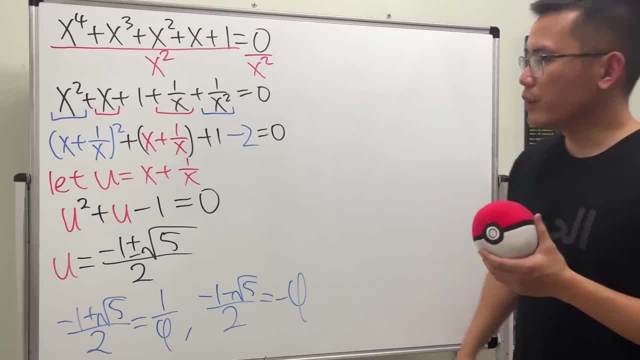 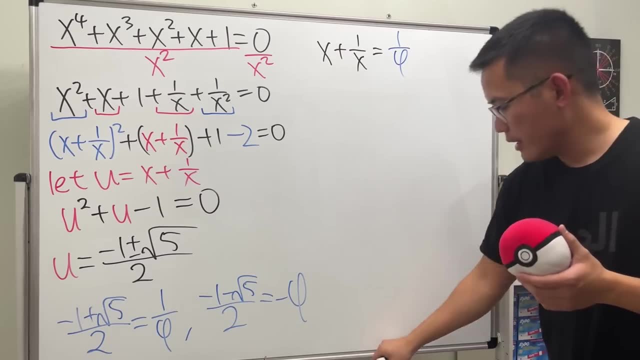 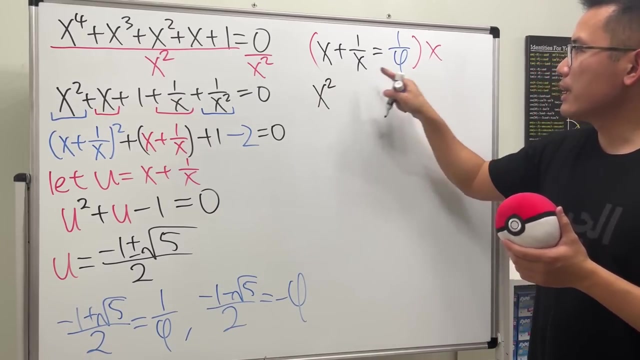 All, right now we know that x plus 1 over x is equal to this or is equal to that, and we'll just solve them separately. And then, right here, I'm just going to multiply everybody by x and we will see this is x squared plus 1, and then that's equal to this. I'm going to move. 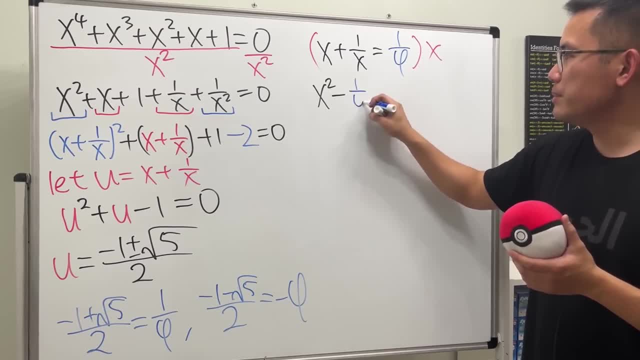 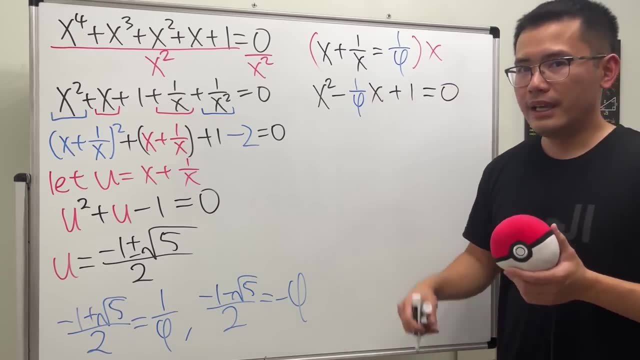 this to the other side, so it becomes negative. and then I will just keep the reciprocal of the ratio and then x, and then the plus 1 here, And that's equal to 0. And to solve this let's just use the quadratic formula again. 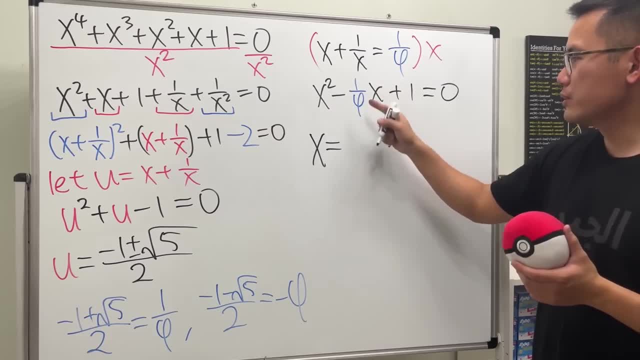 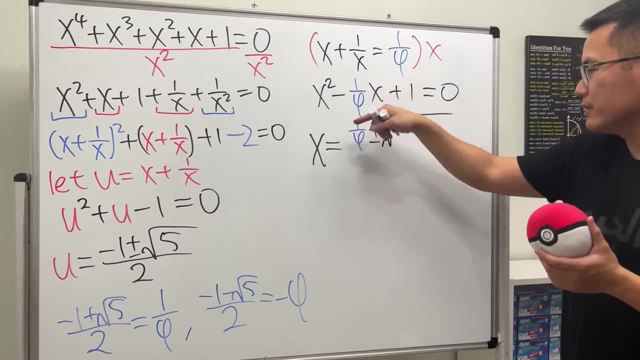 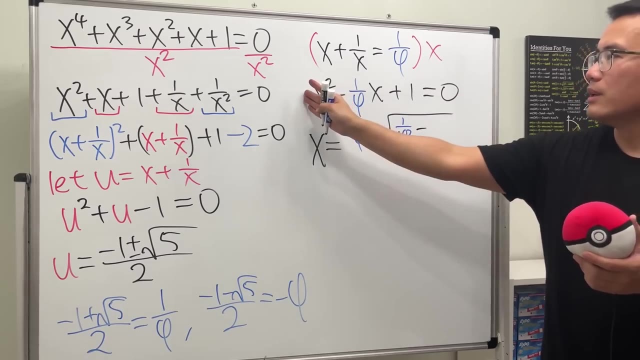 x is equal to negative b, which is going to give us just positive, and then plus or minus square root b squared, Well, that will give us positive. but I'm just going to write it down like this: And then minus 4 times 1 times 1,, which is just minus 4, and then all over 2 times 1.. 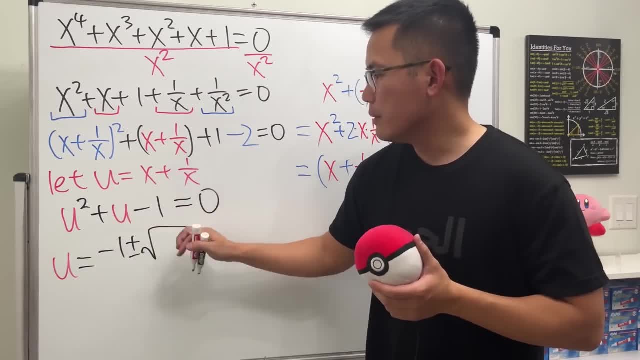 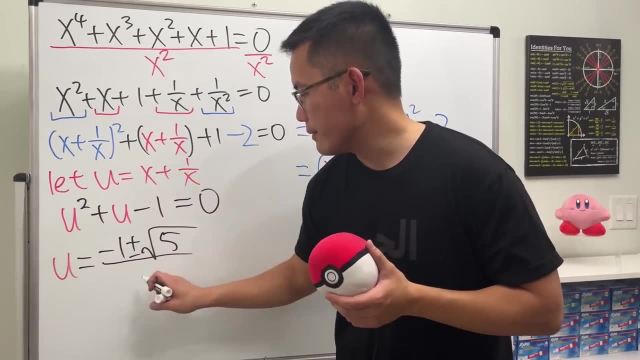 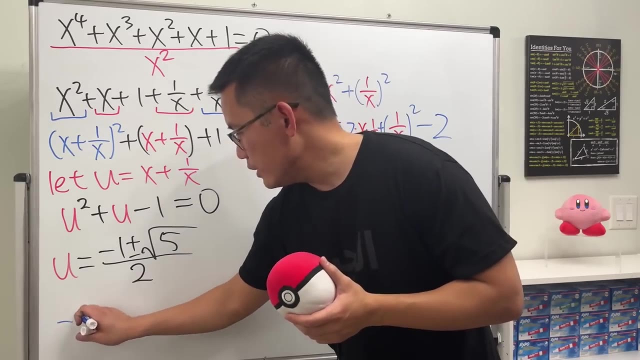 equal to negative 1 of 1 square minus 4 times this and that which is going to be plus 4. so to get this 5 and then over 2 times 1. cool, you know what's cooler? this right here, when we take the positive negative 1 plus. 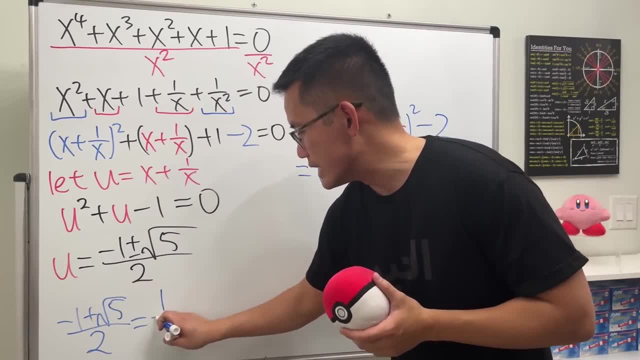 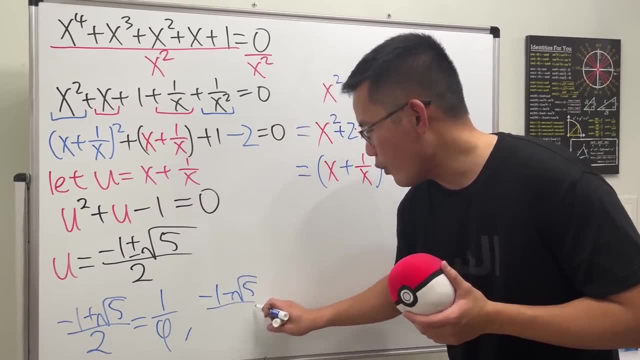 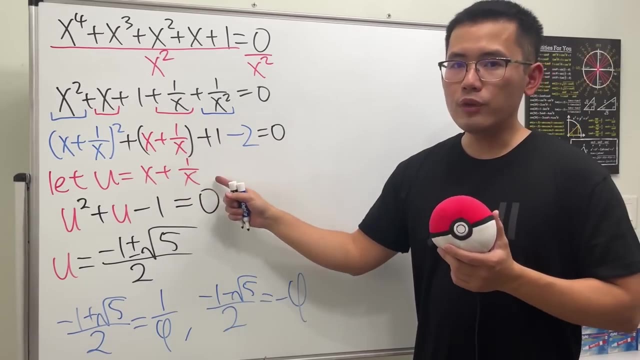 square root of 5 over 2. this, right here, is just the reciprocal of the golden ratio, and when we take the negative, we will get negative 1 minus square root of 5 over 2, and this, right here, is just a negative golden ratio. all right, now we know that x plus 1 over x is equal to this or is equal to that, and we'll just 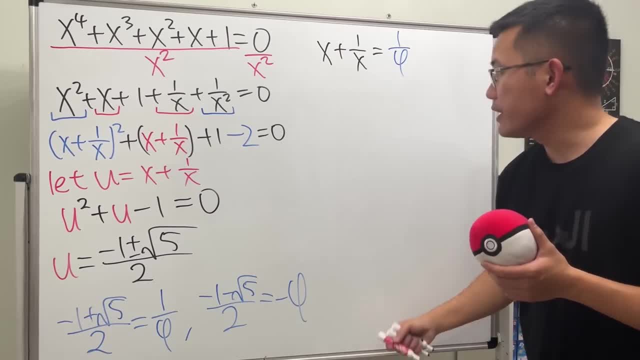 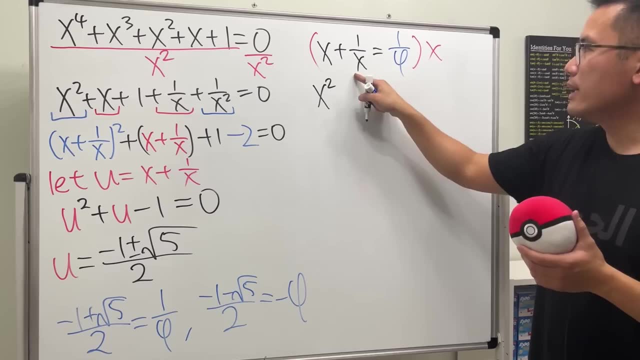 solve them separately. and then, right here, i'm just going to multiply everybody by x and we will see this is x square plus 1, and then that's equal to this. i'm going to move this to the other side so it becomes negative, and then i will just keep the reciprocal of the golden ratio. 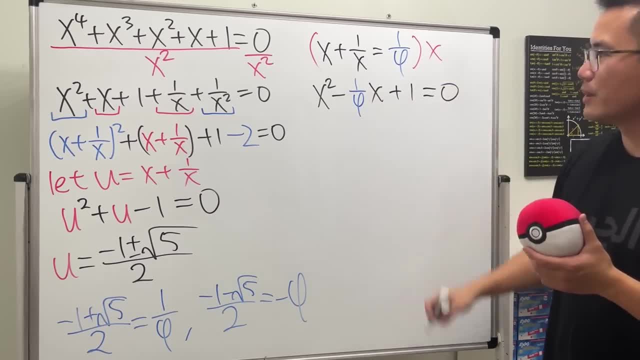 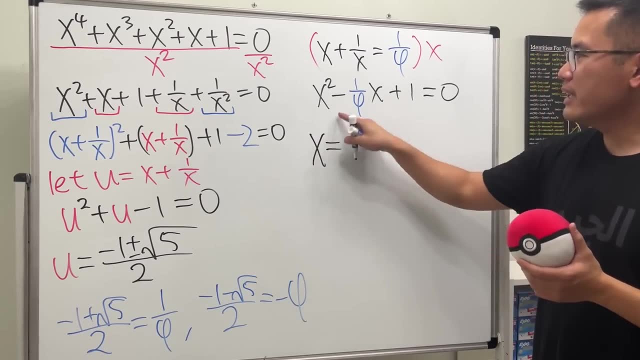 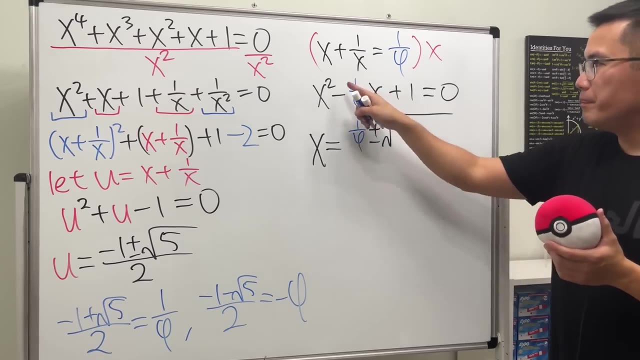 and then x, and then the plus 1 here, and that's equal to 0. and to solve this let's just use the quadratic formula. again, x is equal to negative b, which is going to give us just positive, and then plus or minus square root, b square. well, that will. 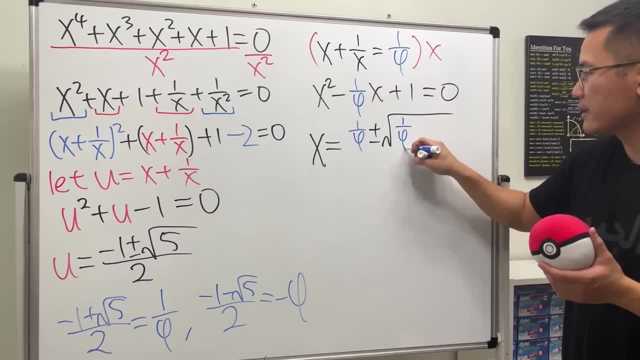 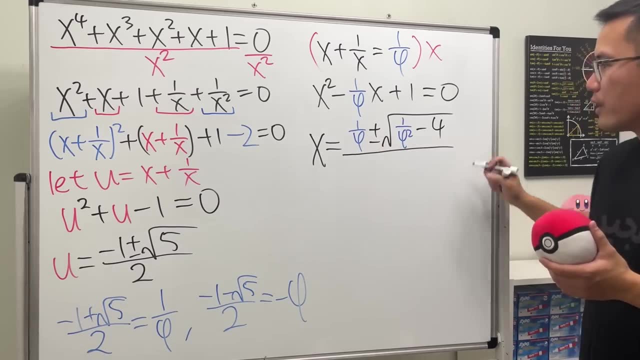 give us positive. but i'm just going to write- yeah, i'm just going to write it down like this- and then minus 4 times 1 times 1, which is just minus 4, and then all over 2 times 1.. so, from here, 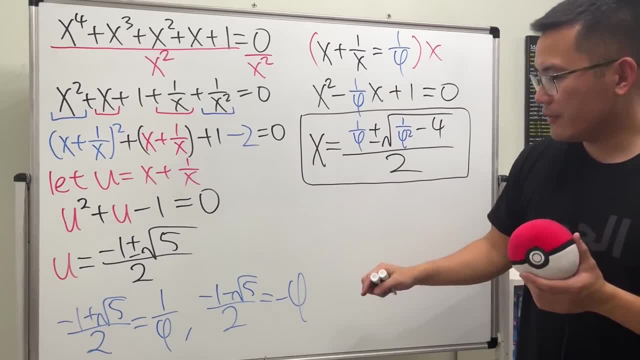 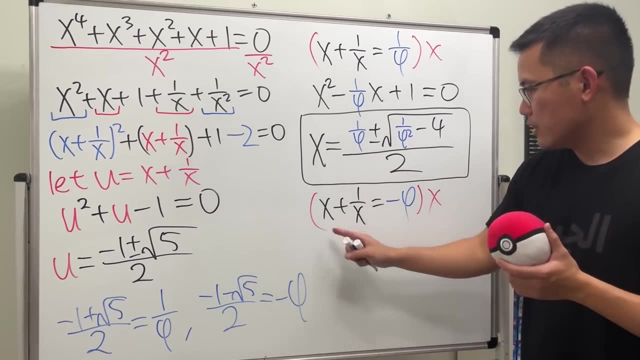 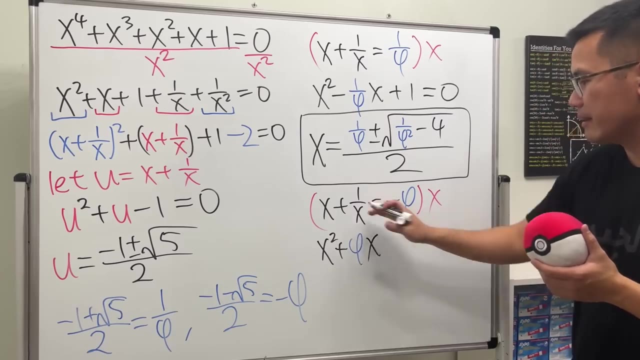 we have two answers, and then we will also have the negative golden ratio part. and then, right here, let's just multiply everybody by x again, so we have the x squared and then plus phi times x, and then plus 1, and that's equal to 0. use the quadratic formula again. 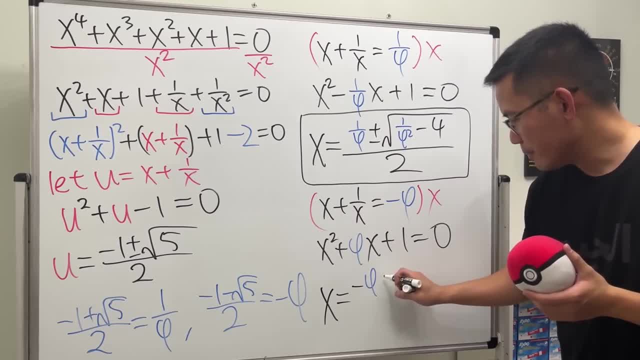 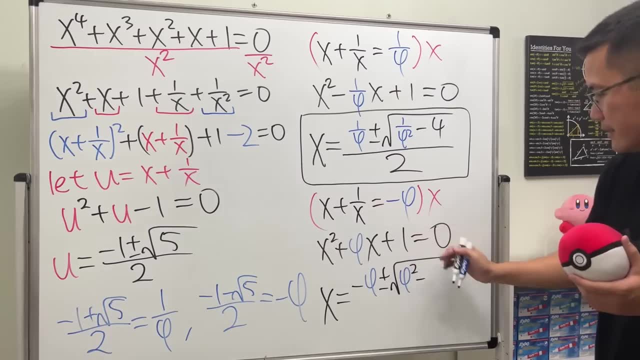 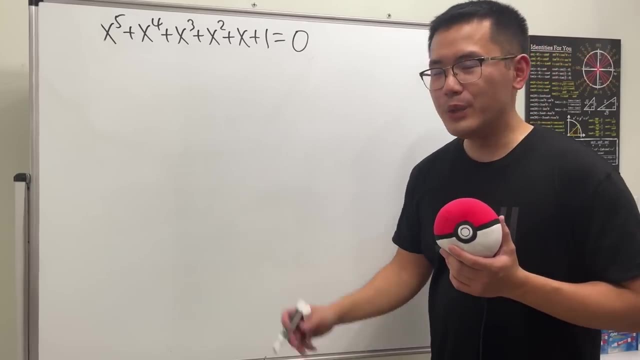 x is equal to negative, v plus or minus square root, and then we have the v Square, and then minus 4 times this and that, which results in minus 4, or over 2.. Excellent, Level 5.. Finally, we have this quintic equation and of course I'll show you guys the quintic formula. 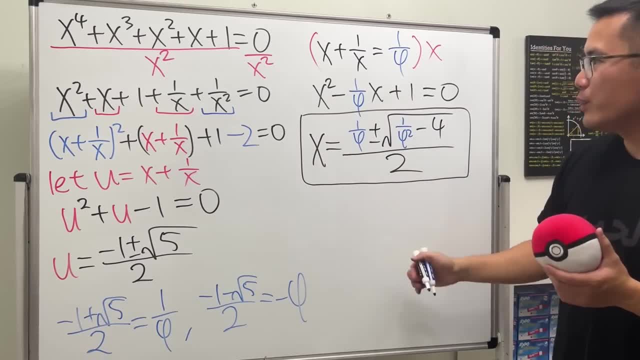 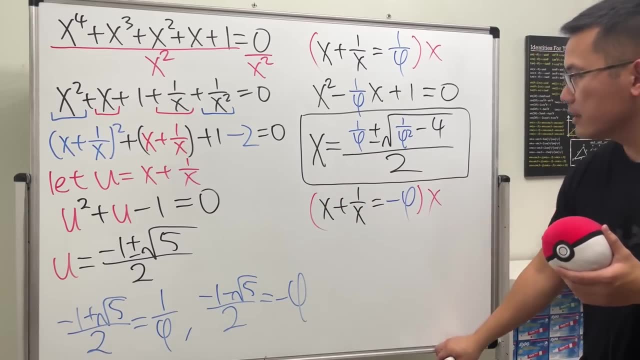 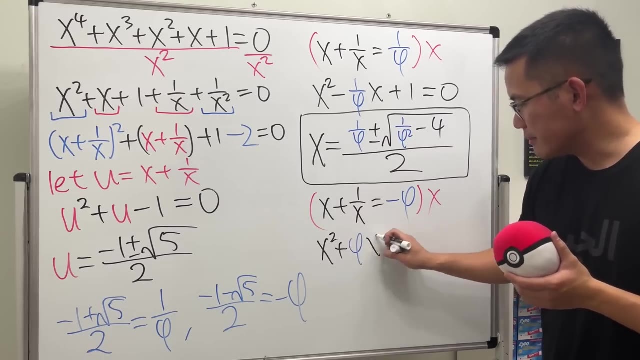 From here we have two answers, And then we will also have the negative golden ratio part. And then right here let's just multiply everybody by x again, So we have the x squared and then plus phi times x, and then plus 1, and that's equal to 0.. 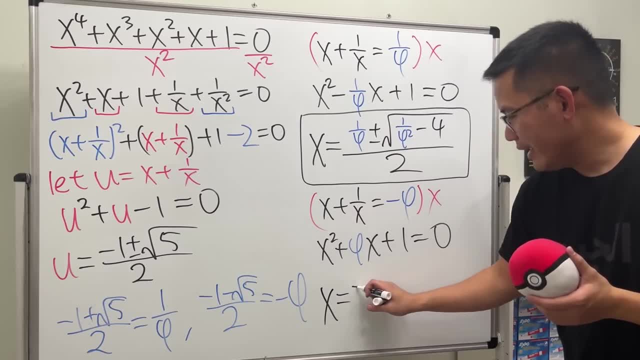 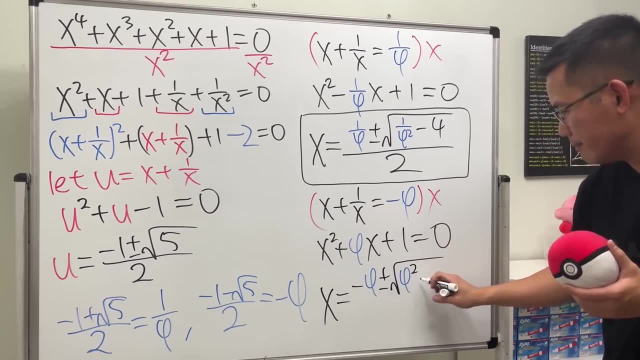 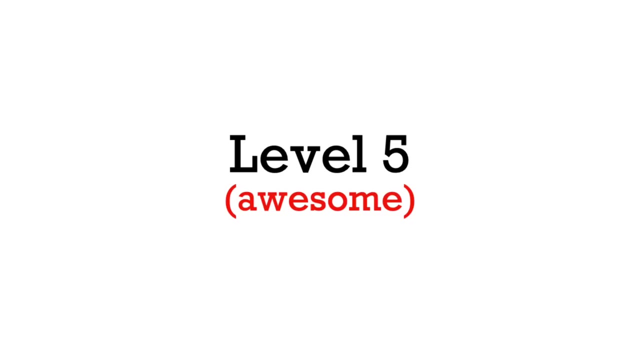 Use the quadratic formula again: x is equal to negative phi plus or minus square root, and then we have the v square, and then minus four times this and that which is minus four or over two, excellent level five. finally, we have this quintic equation and of course i'll show you guys the quintic formula. 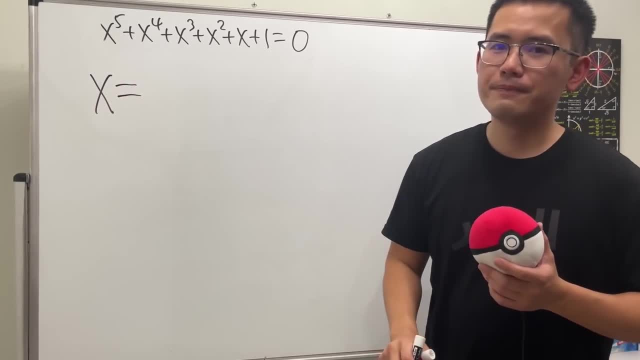 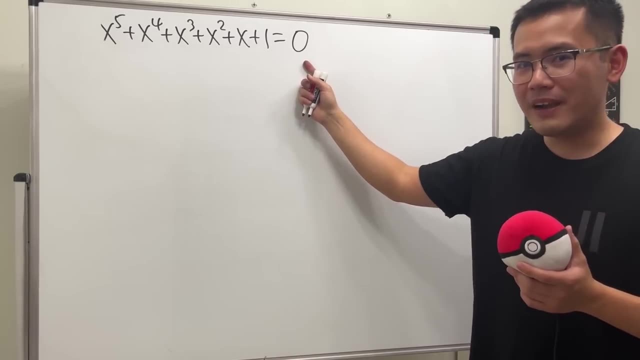 which says x is equal to just kidding. unfortunately there's no such a formula and in fact for this equation we can solve it by factoring, by grouping the first three terms and then the last three terms, and we can go from there. but we did that earlier, so i'll show you. 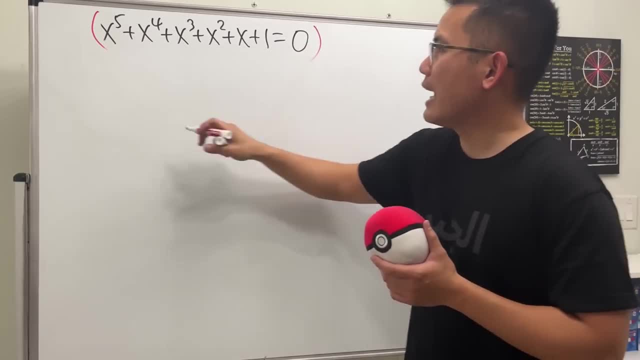 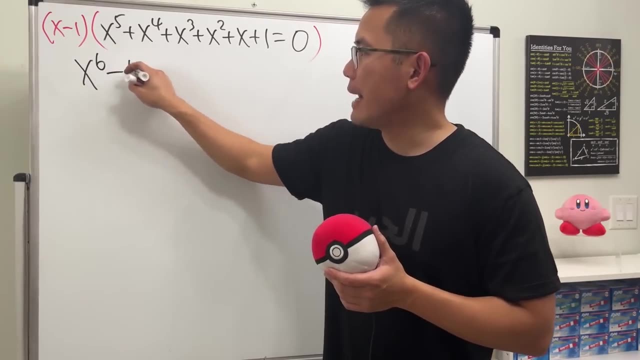 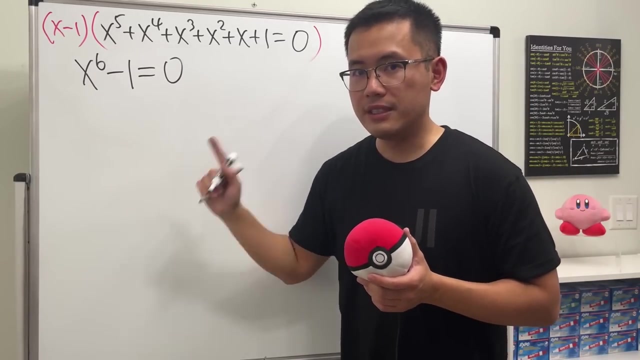 get something else. let's actually multiply this equation by x minus one. when we multiply the left hand side, we'll just get x to the six power minus one, and then the right hand side will still give us zero. however, notice that, though, this equation has a total of six solutions, but originally we 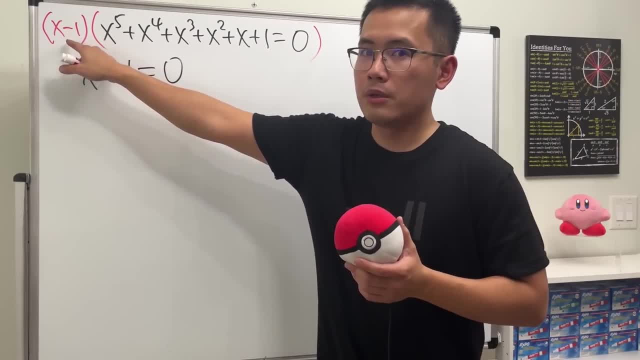 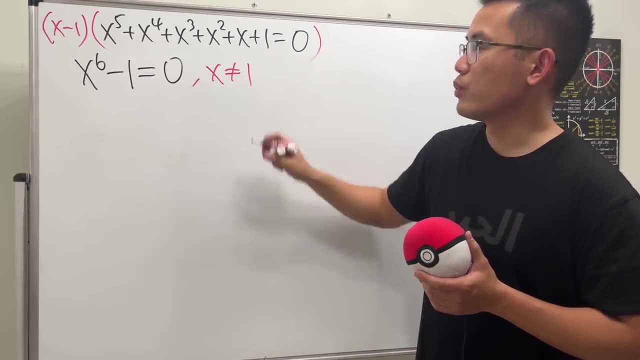 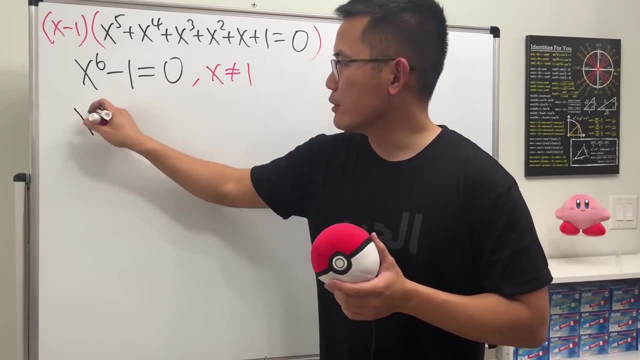 only have five, and the reason is because we multiply out an extra factor. so we just have to indicate that. look at this, but x cannot be equal to one. all right, and now? what's so good about solving this? well, we can move this to the other side, so we just have to. 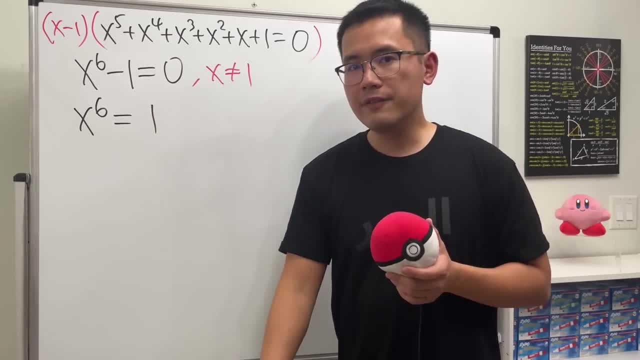 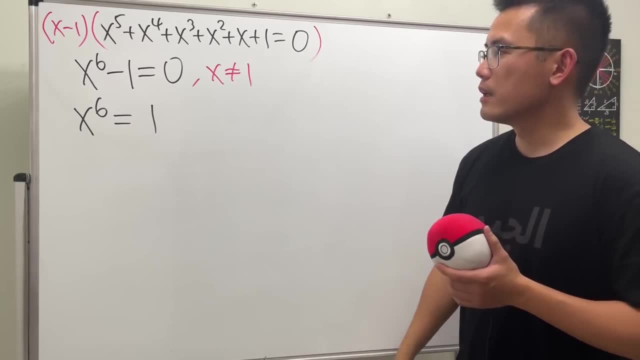 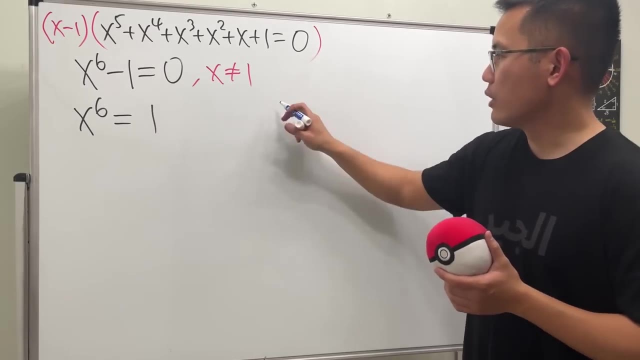 look at x to the sixth power is equal to one. in fact, we're just trying to find all the sixth root of one, but we are not going to count x equal to one as a solution, and to do so we can utilize complex numbers. take one to the complex world, so i'll. 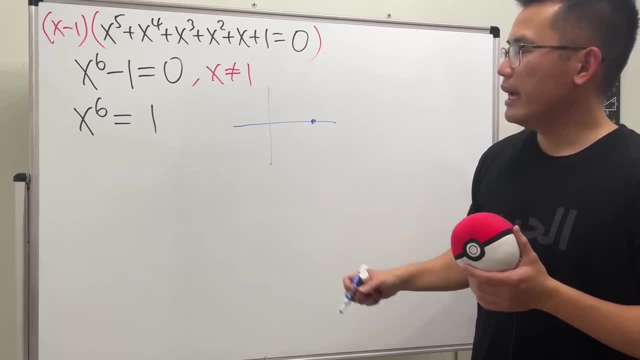 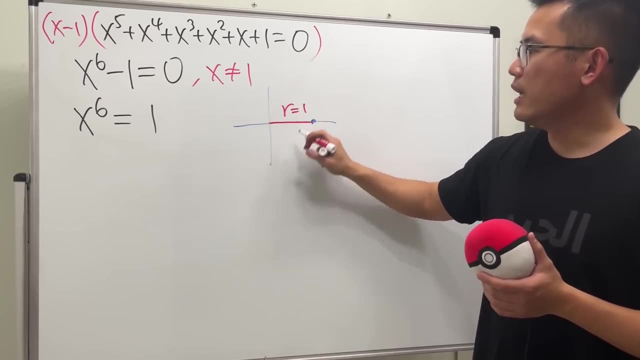 put that down right here for you guys- one is right here- and then write this in the polar form. we need two things. the first thing is the distance from the origin to here, which is just one, and then the next thing is the angle. by looking at this, the angle is zero. however, we can keep rotating. 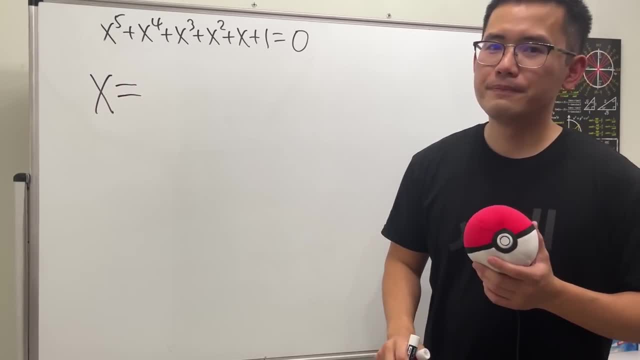 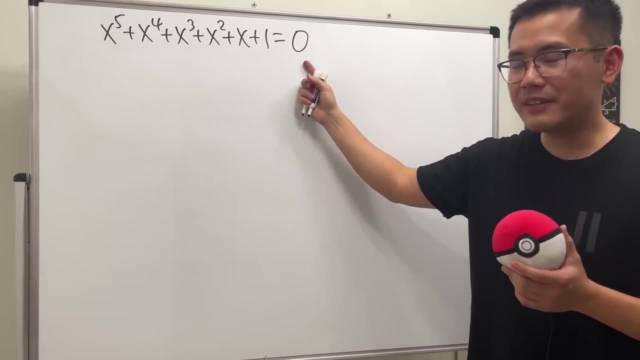 which says x is equal to Just kidding. Unfortunately there's no such a formula And in fact for this equation we can solve it by factoring, by grouping the first three terms and then the last three terms, and we can go from there. 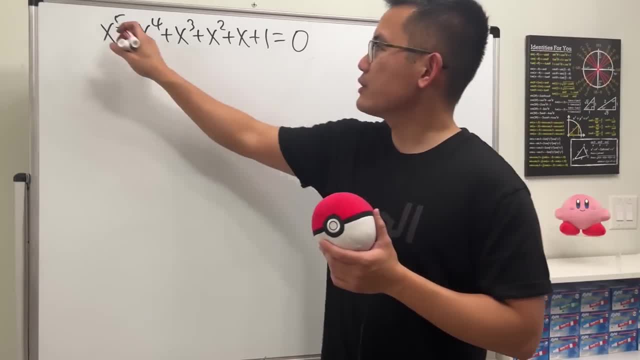 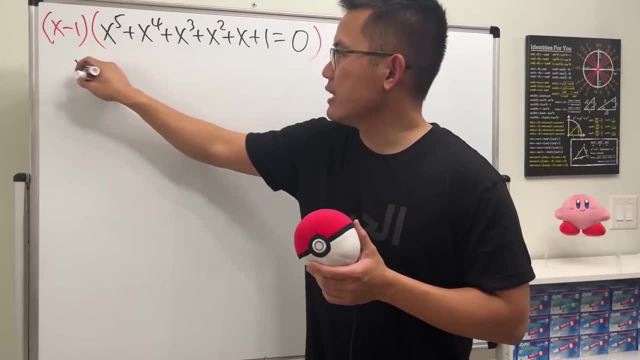 But we did that earlier, so I'll show you guys something else. Let's actually multiply this equation by x minus 1.. When we multiply the left-hand side, we'll just get x to the 6th power minus 1, and then the right-hand side will still give us 0.. 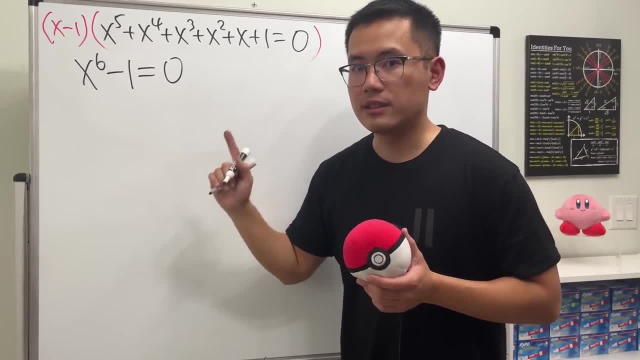 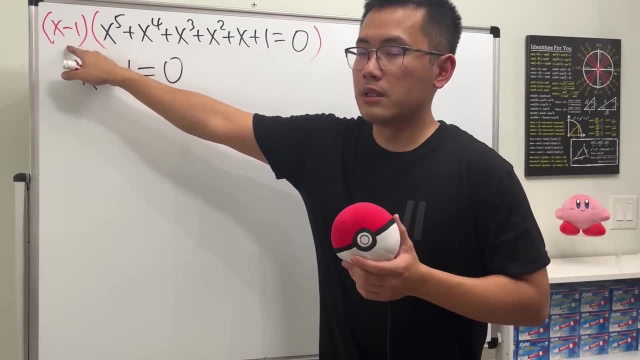 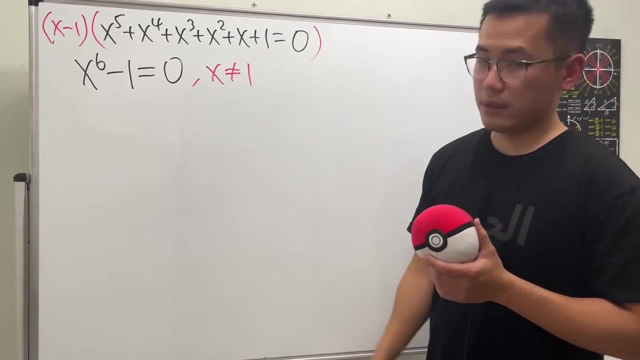 However, notice that this equation has a total of 6 solutions, but originally we only have 5. And the reason is because we multiplied out an extra factor. So we just have to indicate that. Look at this, but x cannot be equal to 1.. 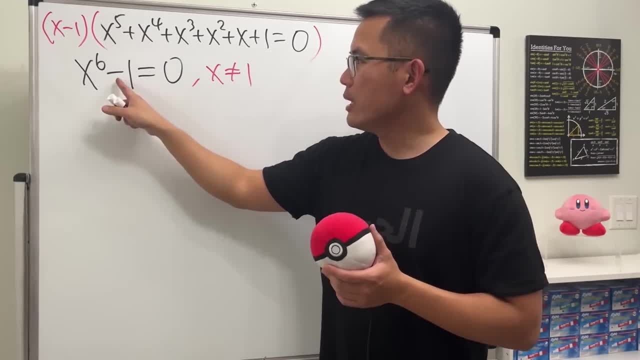 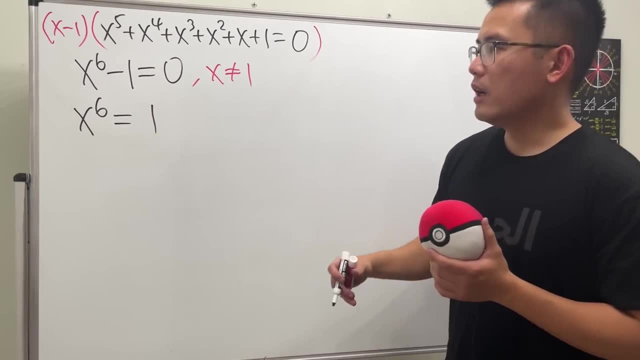 And now, what's so good about solving this? Well, we can move this to the other side, so we just have to look at x to the 6th power is equal to 1.. In fact, we're just trying to find all the 6th roots of 1,. 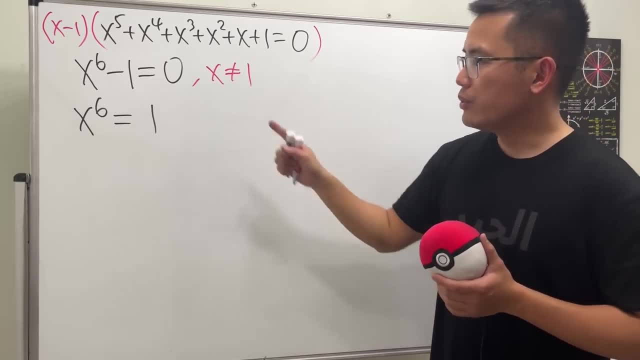 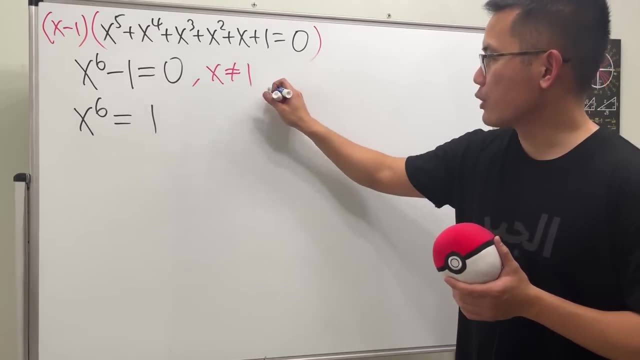 but we are not going to count x equal to 1 as a solution, And to do so we can utilize complex numbers. Take 1 to the complex world, So I'll put that down right here for you guys- 1 is right here- and then write this in the polar form. we need two things. 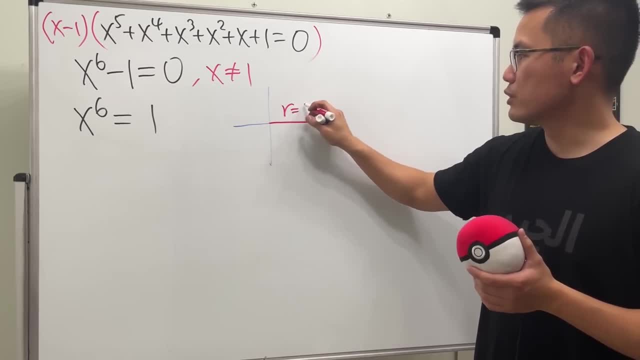 The first thing is the distance from the origin to here, which is just 1.. And then the next thing is the angle. By looking at this, the angle is 0.. However, we can keep rotating 2pi or the other way: 2pi, right. 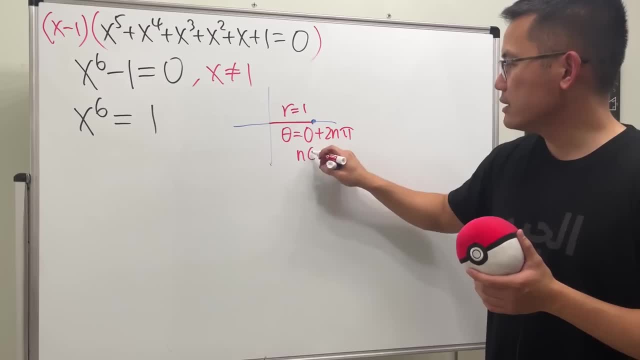 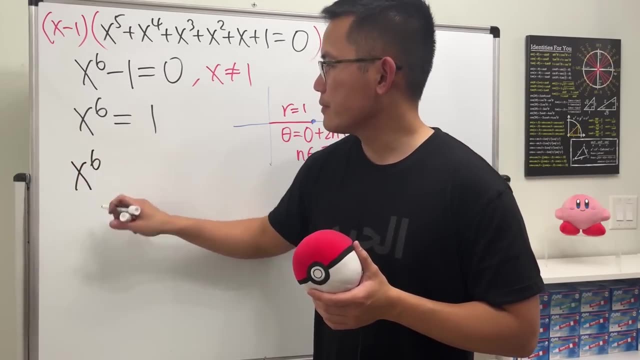 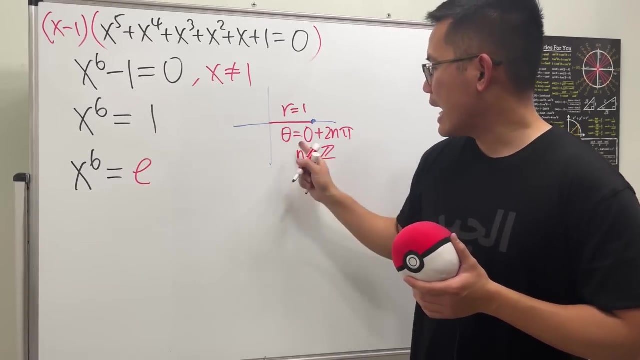 So we just have to add 2pi, where n is an integer. So in fact for the 1,- we can just look at this right here- x to the 6th power is equal to 1.. So it's equal to r is 1, and then we have the e and then i times theta. 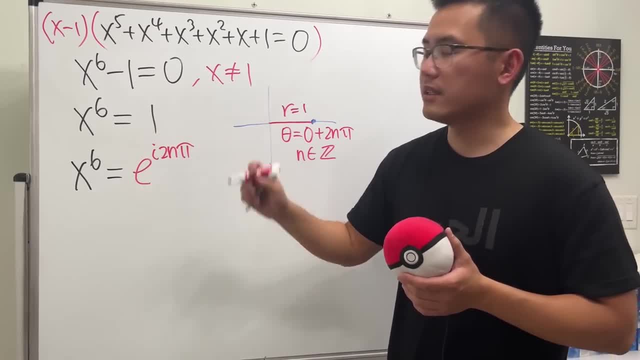 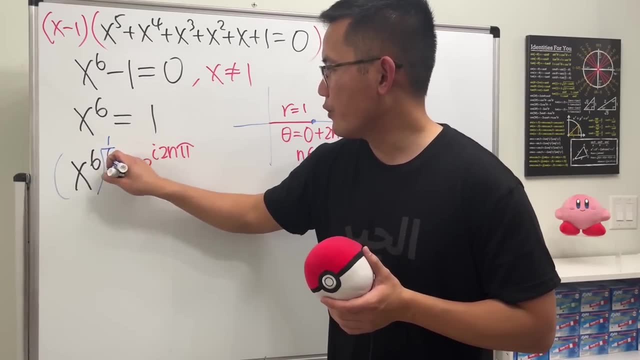 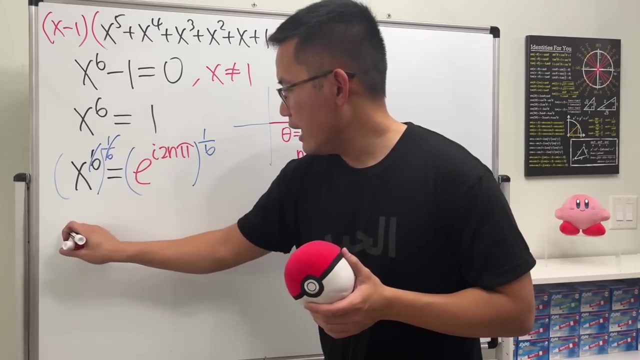 So i times 2pi like this: Now we want to get the x right, So let's just take both sides to the 1 over 6th power, like so And this, and that will cancel. So we are going to get x being equal to. 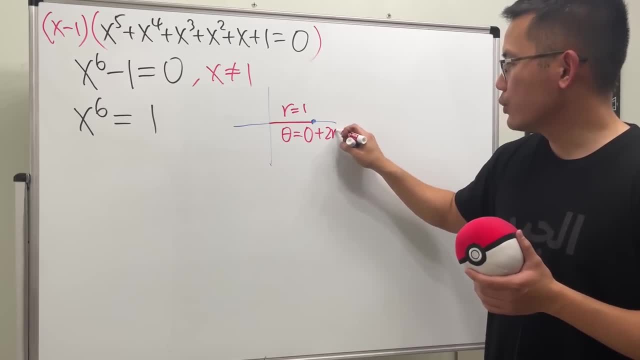 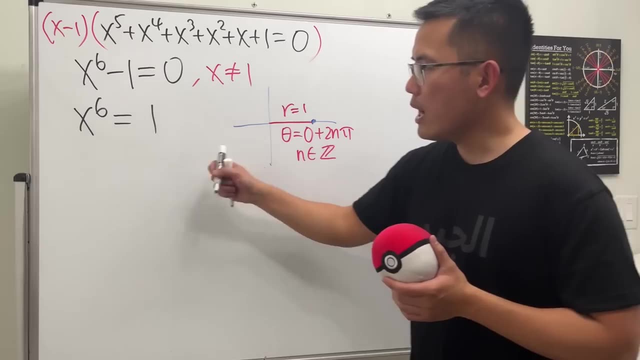 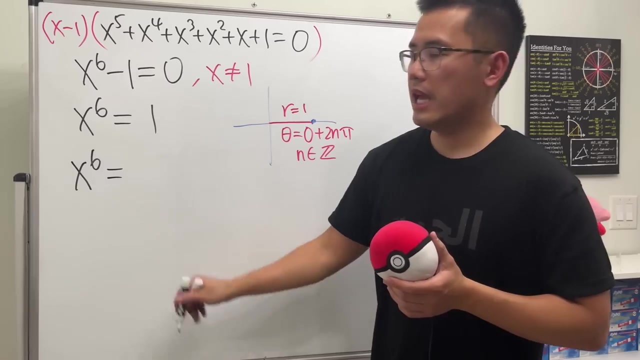 two pi, or the other way, two pi, right. so we just have to add two um pi where n is an integer. so in fact for the one- we can just look at this right here- x to the sixth power is equal to, r is one, and then we have the e, and then i times theta. so i times. 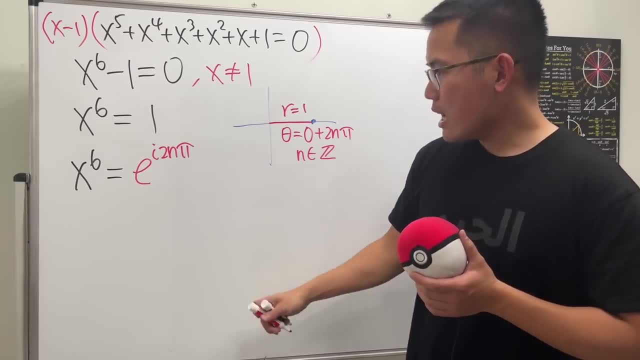 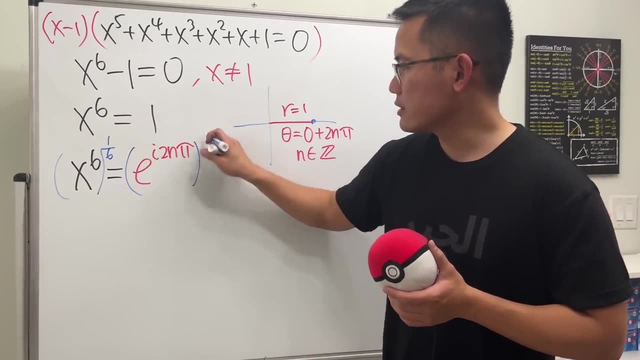 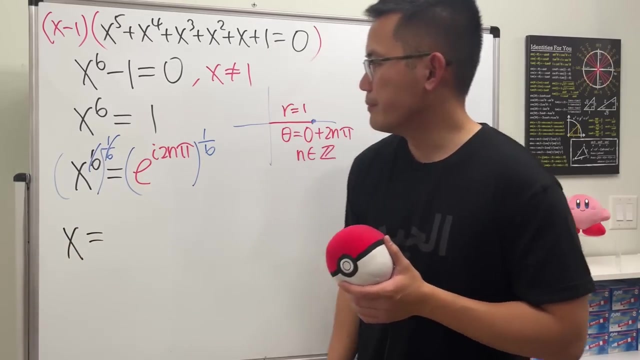 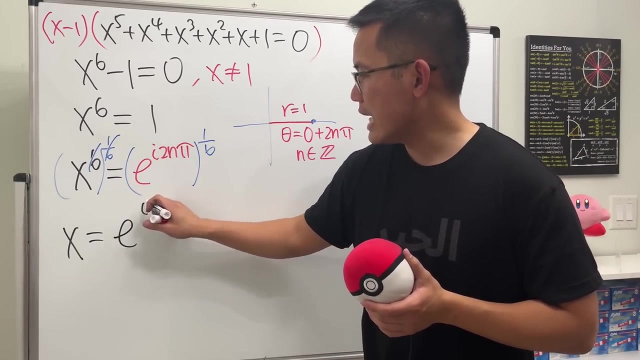 two um pi like this: now we want to get the x right, so let's just take both sides to the 1 over 6 power like so and this, and that will cancel. so we are going to get x being equal to. we can divide, reduce all that stuff. so this is going to be e and then we will just have i and then m pi over 3. 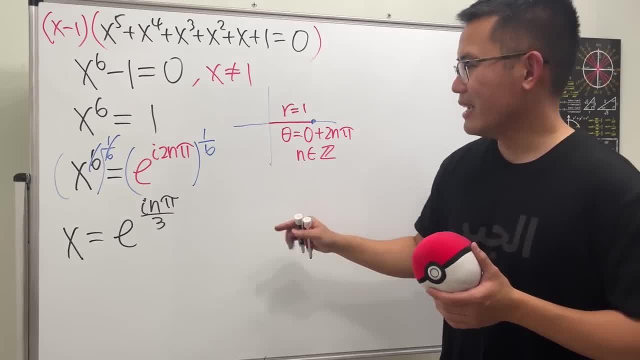 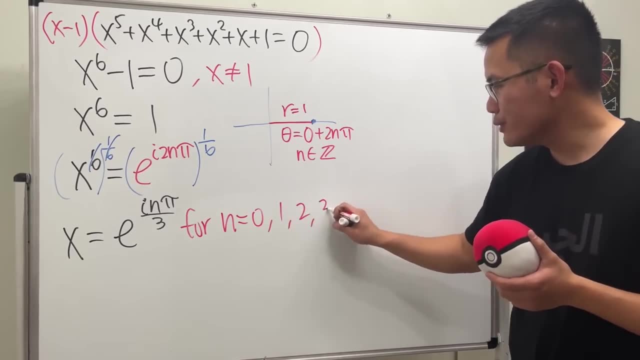 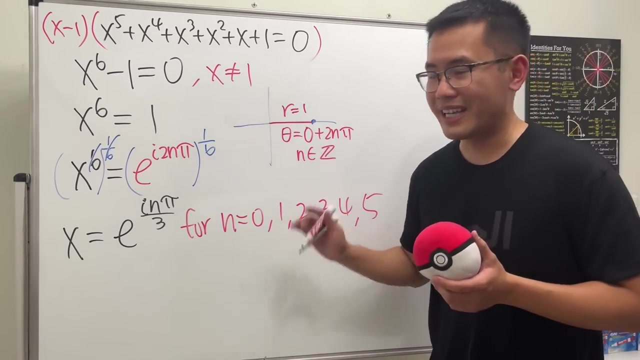 but what the ends, though? well, keep this in mind. when we want to find the sixth root of one, all we have to do is plug in: n is equal to zero. one, two, three, four, five, and that's it. if you continue, they will just give you duplicate the answers from here. so don't do that. and right here. 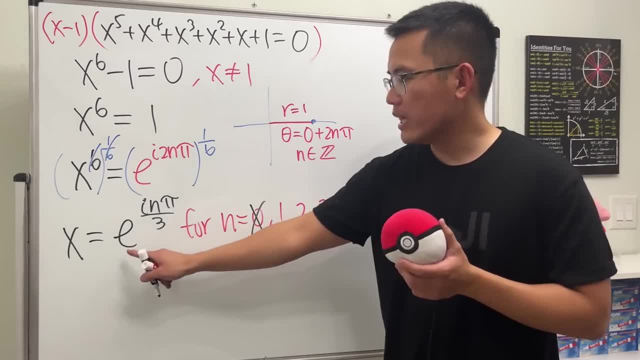 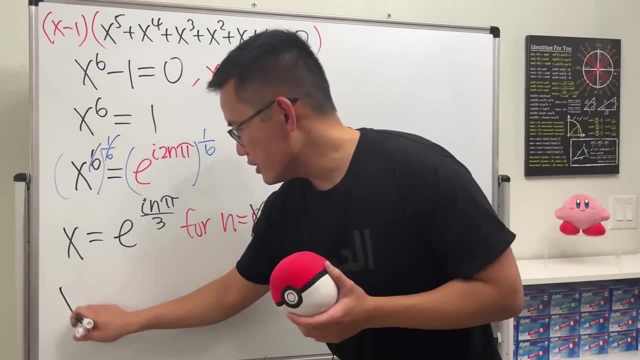 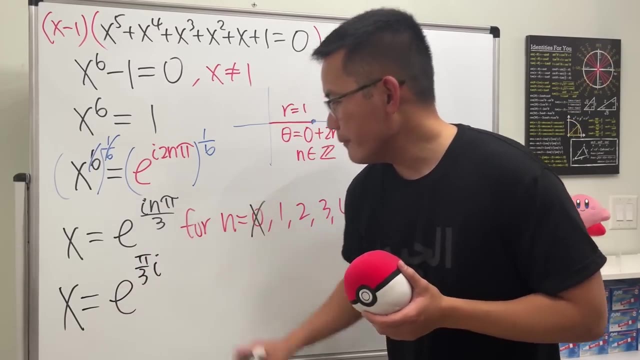 you will see that we are not going to use zero, because if so, we will get e to the zero's power, and that's one. and we say: x is not equal to 1.. so now we just have to plug in this right here. so, ladies and gentlemen, x is equal to plugging 1 into n. we will get e to the pi over 3, i and of. 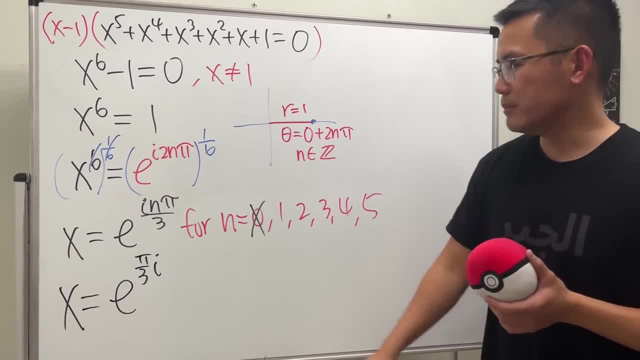 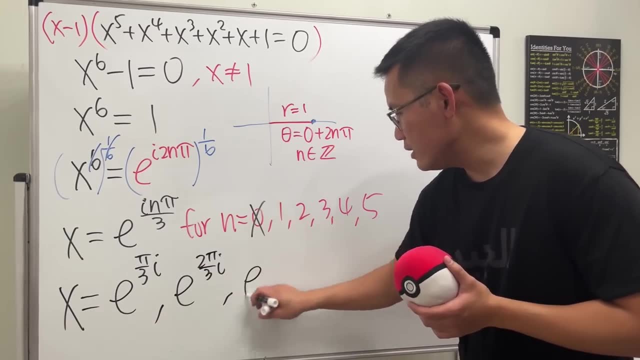 course you can use the euler's formula to write the expression in the standard form, but i'm just going to leave you like this: and then next we will have e to the 2 pi over 3 i, and then e to the three- pi over three, which is just pi, and then i, which is actually just negative one. 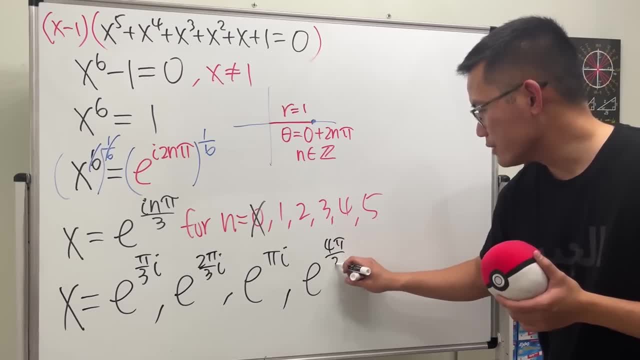 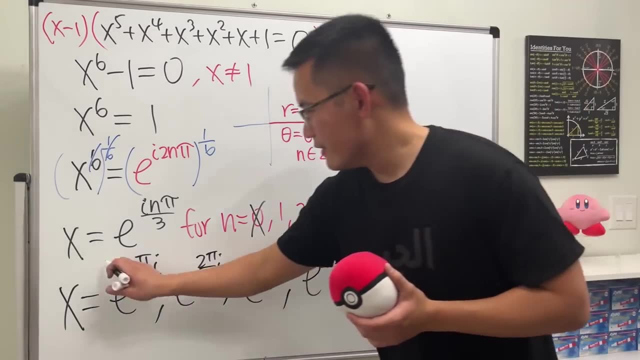 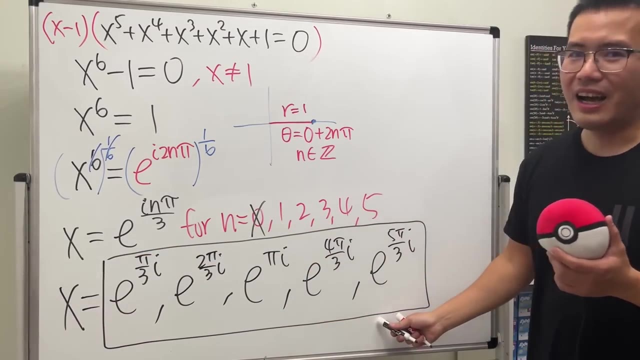 and then e to the four pi over three i and lastly, e to the five pi over three i. all right, very, very cool. here are the five solutions to the original equation- awesome.